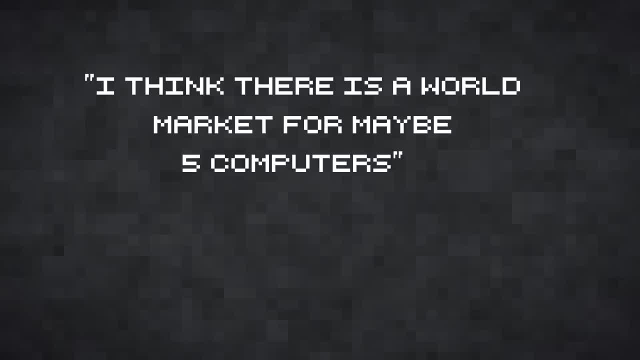 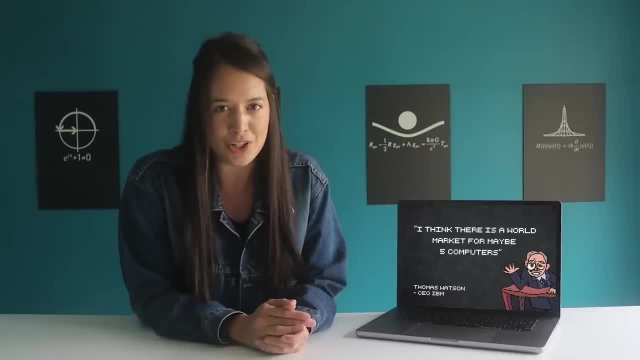 I think there is a world market for maybe five computers. This quote is attributed to Thomas Watson, long-time CEO of IBM. There's no doubt this prediction turned out completely wrong, But why? Let's figure it out by looking at some of the earliest computing devices. 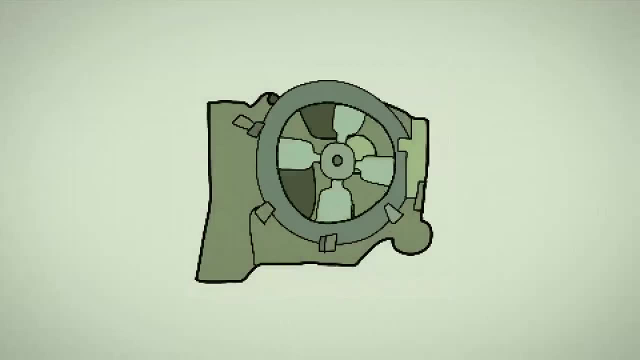 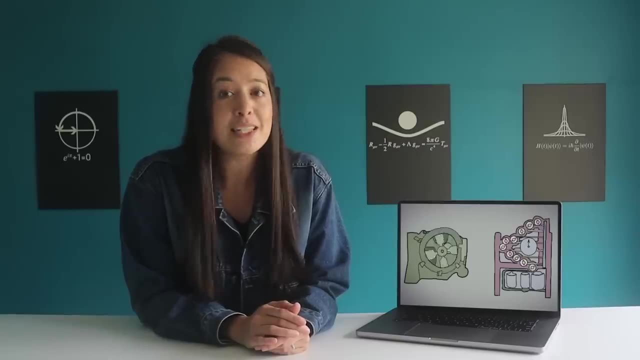 Like this thing used to calculate the motions of the moon and sun, Or this one used to predict the motion of the tides. They were very good at the job they were designed to do, but they didn't receive the attention and faith. 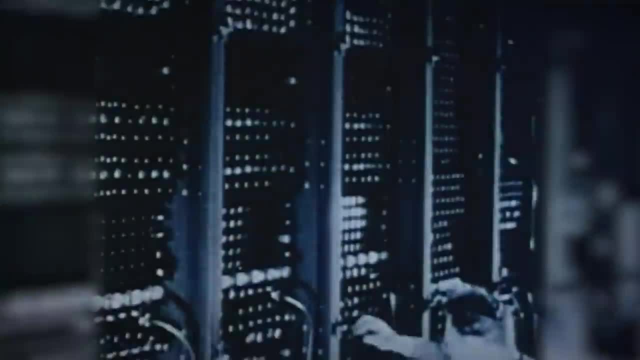 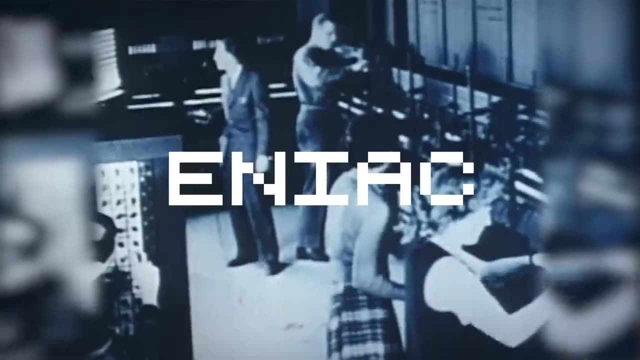 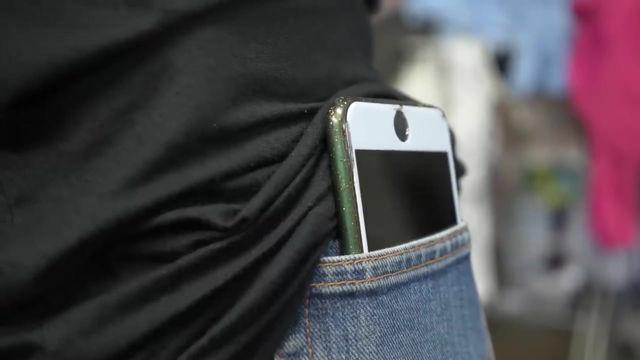 Why not The first modern digital computer ever built? ENIAC was created for the sole purpose of computing artillery firing tables. But unlike these other devices, ENIAC's descendants went on to rule the world to the point where nearly everyone carries one in their pocket. 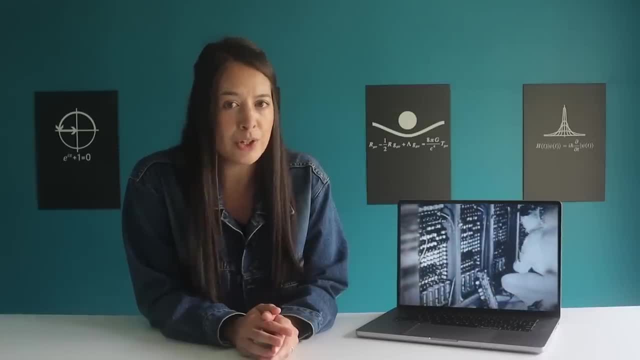 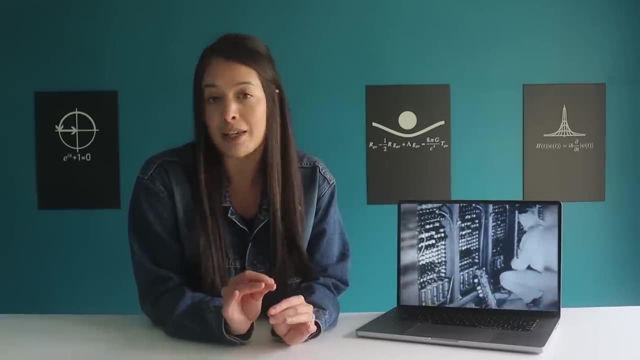 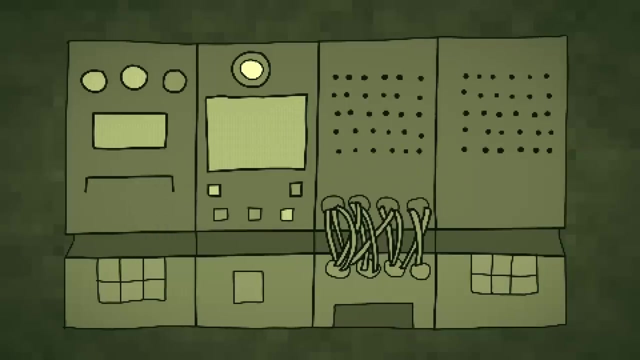 What was different about ENIAC? What could it do that computing devices before it couldn't? The secret source was that ENIAC could be programmed. programmed, This meant you could make it behave differently by putting in different instructions. Programmed with the right set of instructions, ENIAC could act like the device that predicted. 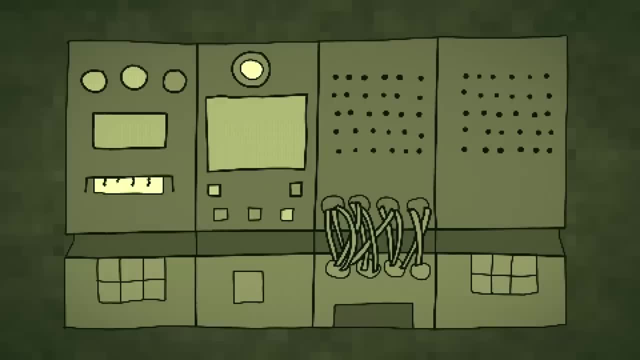 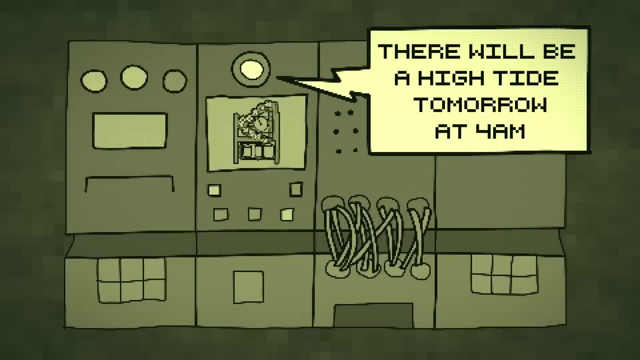 the motions of the sun and moon, Program it with a different set of instructions and it could act like the type-predicting device, In fact, any program that any computer could run. ENIAC could run, at least in theory. 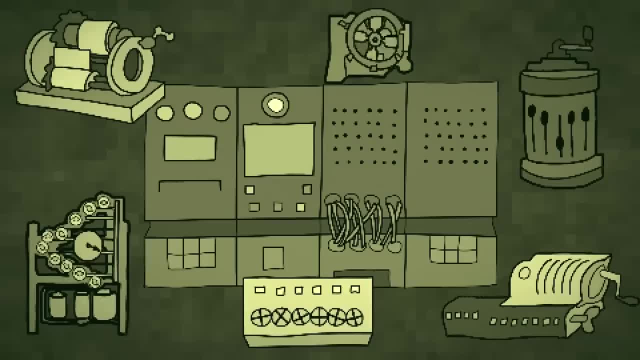 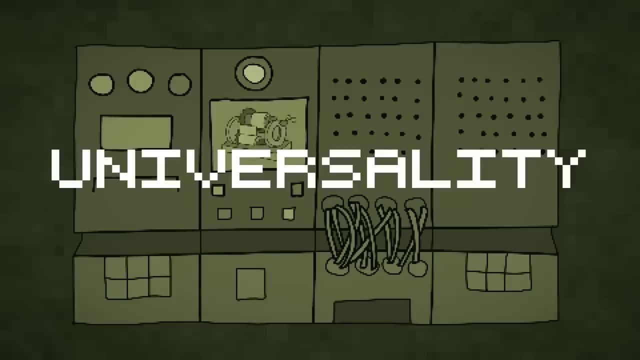 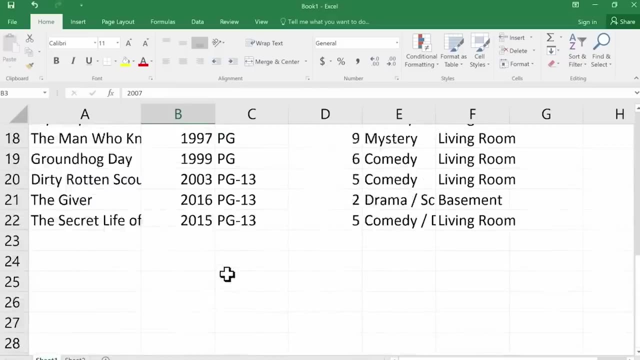 Rather than having to build a new machine for every purpose, you could just switch out instructions. This shape-shifting ability is called universality, and it's the reason for the incredible success of the modern computer. We're so used to it today that we take it for granted, but it truly is incredible. 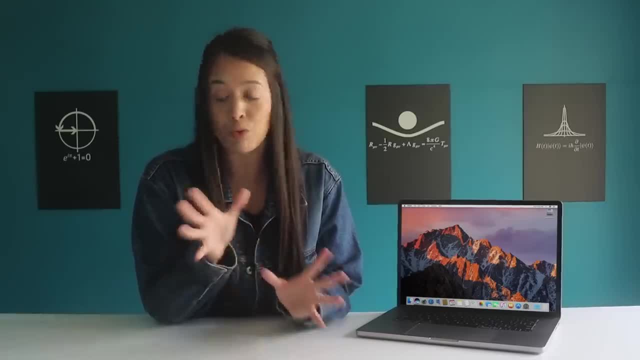 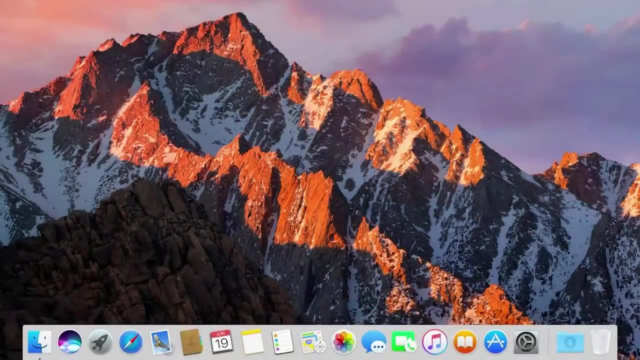 A consequence of universality is that we can have programs running other programs. Just look at your computer's operating system. An operating system is a program, and any time you open Word, play a movie or paint a picture, that's a program running another program. 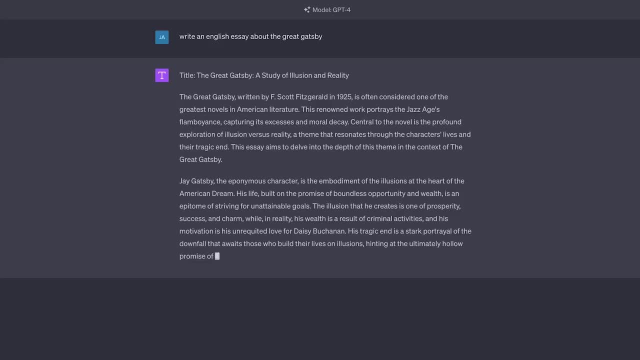 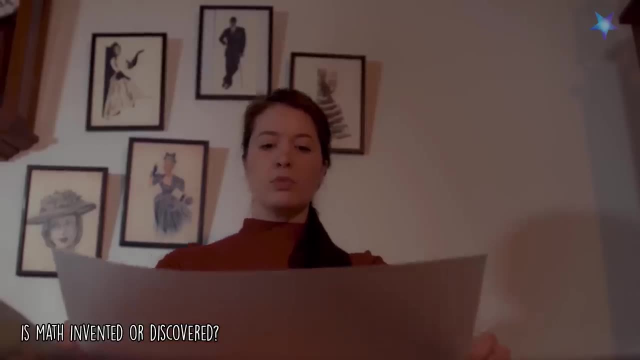 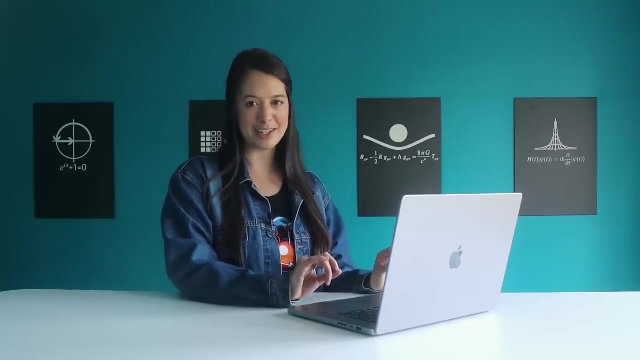 Today, programs have robots roaming around Mars writing English essays and helping doctors make diagnoses. Something else you can do on your computer is watch this documentary I made on our exclusive streaming service, Nebula. Before we continue with the rest of the video, I'd like to tell you about today's sponsor. 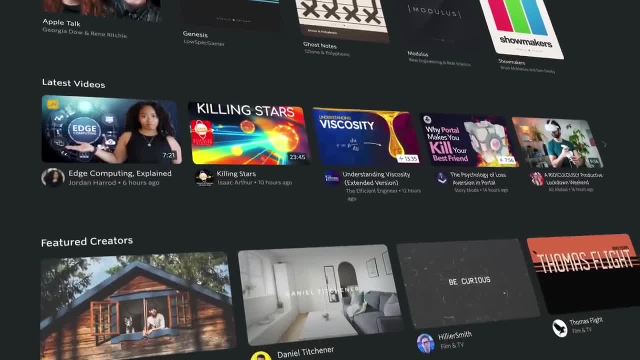 Nebula, Some creative friends and I teamed up with our own streaming platform where we don't have to worry about the pressure of the YouTube algorithm or click-bait titles to keep creating. Nebula is a place where we can focus on passion, projects, experiments and more. 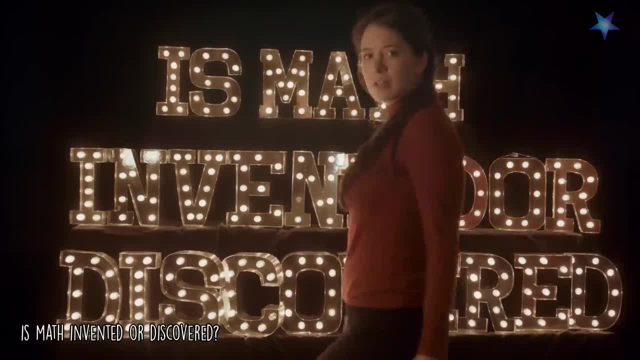 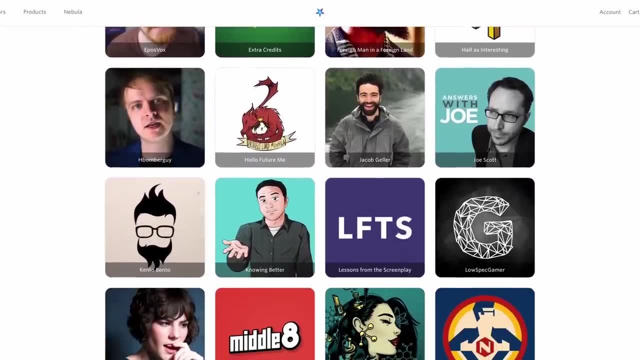 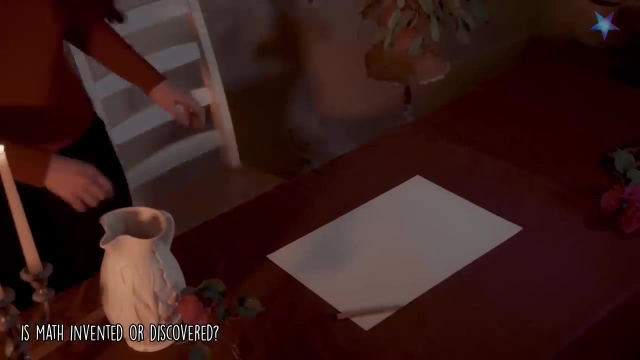 Nebula is a place where we can focus on passion projects, experiments and more. Nebula is a place where we can focus on passion projects, experiments and more If you're a deep thinker and we like to contemplate the boundary between math and 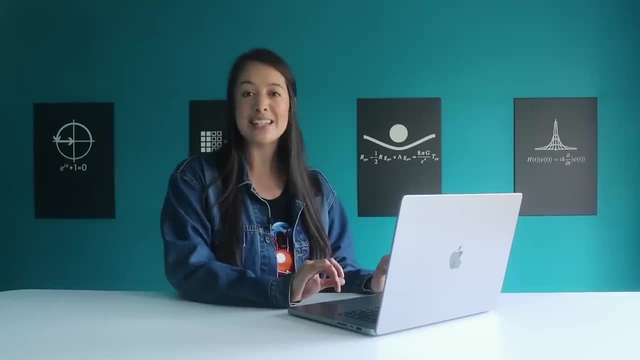 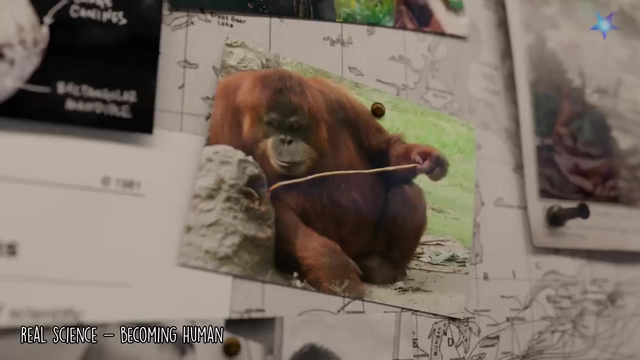 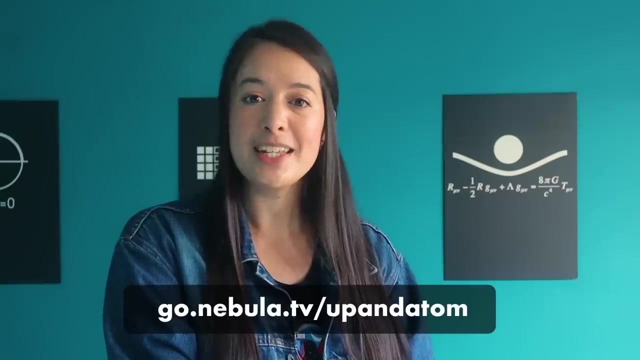 philosophy. I think you'll like my documentary. There are a series of exclusive content on there as well, like Reel Science's amazing new documentary series about the key moments in our human evolution. support this channel and the entire educational community if you sign up using the link on screen. 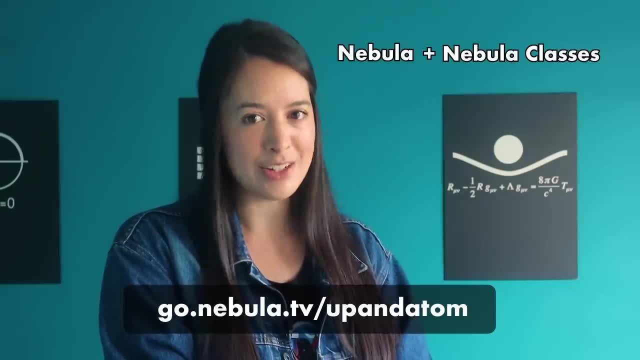 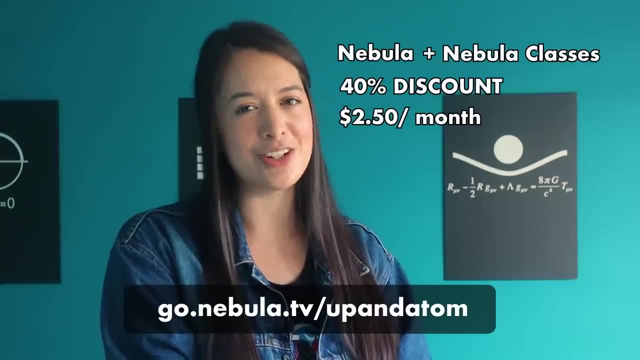 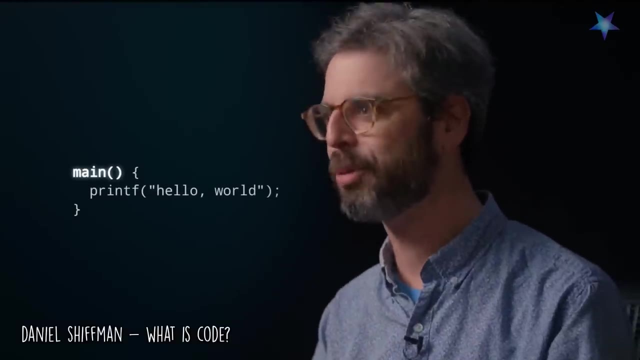 and in the description you'll get both nebula and nebula classes with a 40 discount off the annual plan. that's just a little over 2.50 a month for exclusive high quality educational content made by your favorite creators. nebula classes are where creators make classes about how they do what they. 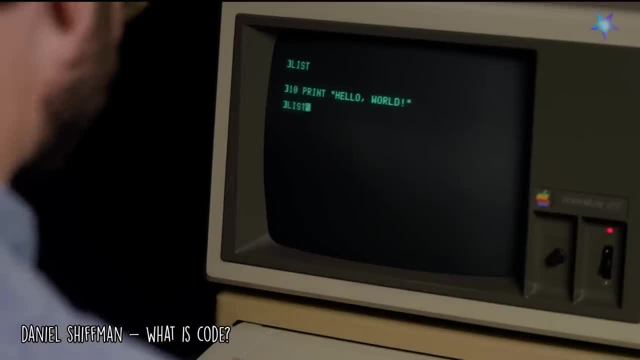 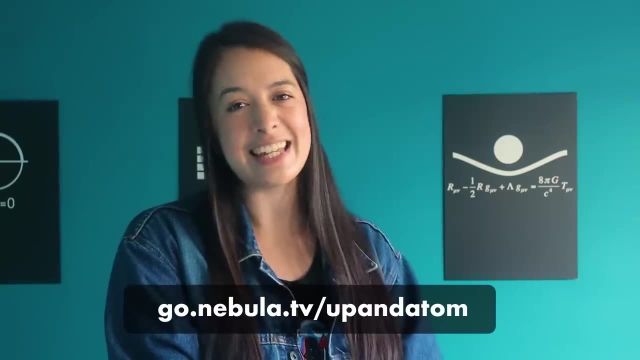 do best. one i highly recommend is what is code? taught by the coding trains daniel schiffman. it's a beginner-friendly introduction to the ins and outs of coding. thank you for listening and thank you, nebula, for sponsoring this episode. speaking of mathematics and coding with the 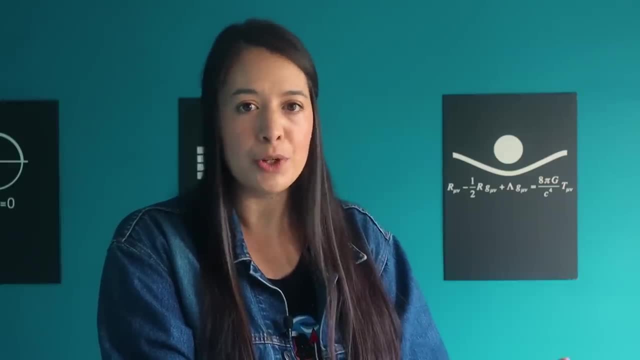 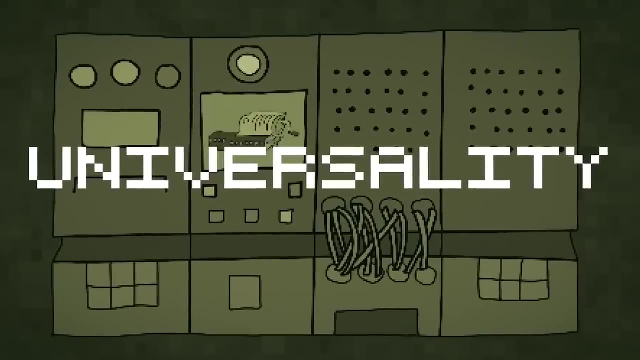 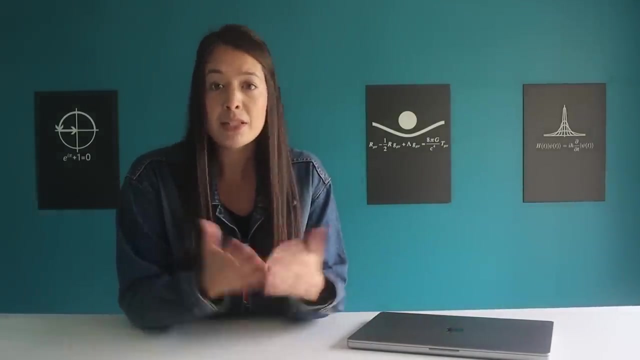 way things are going, it's not hard to imagine that in a few years computers will have solved all of mathematics problems. but in fact this property of universality has a flip side. there are some problems computers will never solve, even in a million years. sometimes seemingly simple. 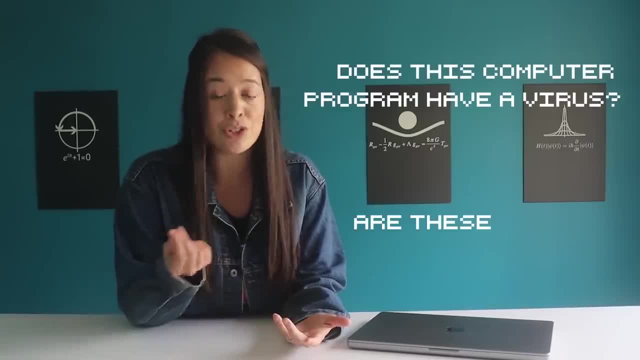 problems like: does the pictures support the idea of龍? all of cycles layer is basically the same problem. extreme problems, import program concept board does what it does at olsun. they deal with values. computer program have a virus, or are these two real numbers equivalent? But wait, how could we? 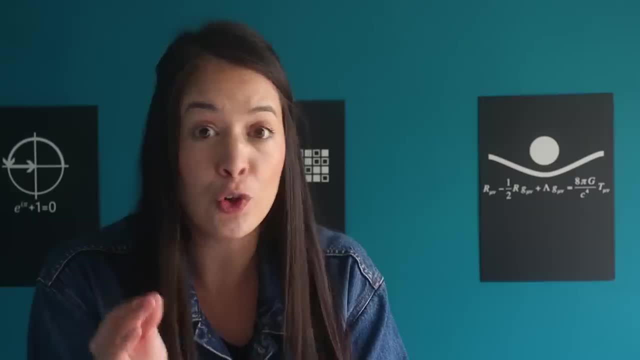 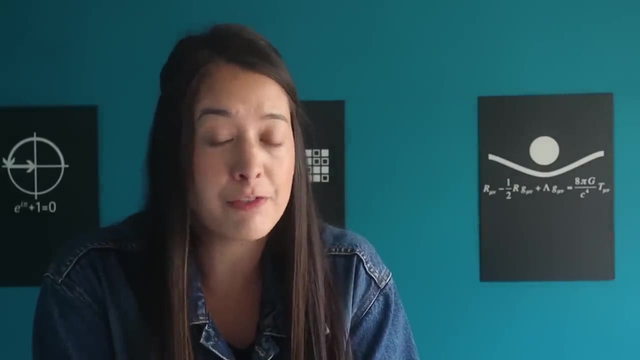 possibly know that. Isn't it a bit arrogant to claim that we know for sure that a computer will never solve some problems? Mathematicians were working on Fermat's last theorem for 358 years before Andrew Wiles solved it. An example even more relevant to this video is the four color. 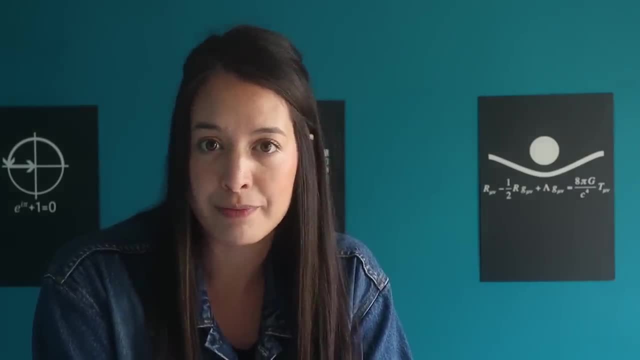 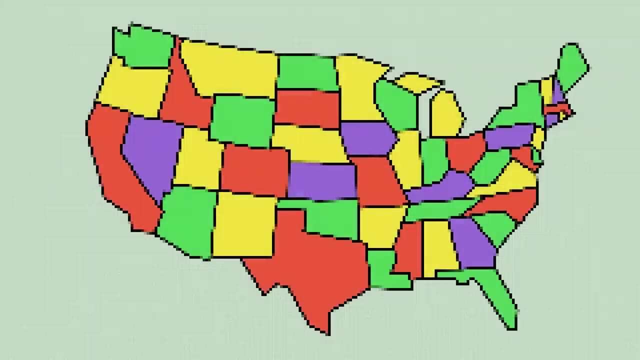 theorem, one of the first computer assisted proofs. The four color theorem states that only four colors are needed to color in any map so that no two adjacent regions have the same color. Mathematicians were working on this for 124 years, before invoking the help of a computer. 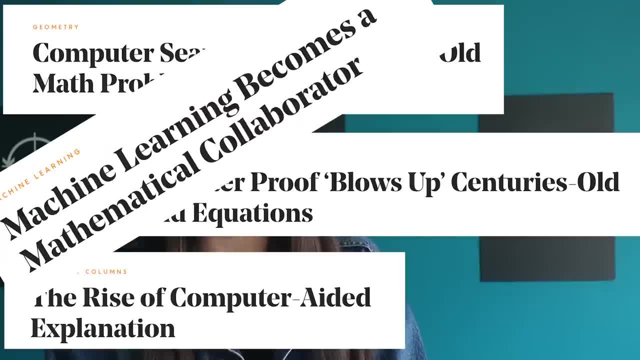 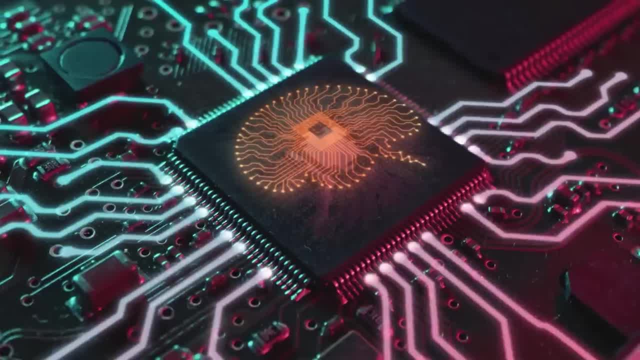 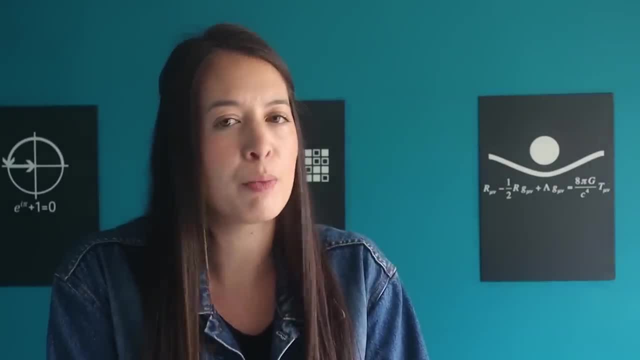 to finally solve it. Today, computer assisted proofs are commonplace. One could argue that, with tools like ChatGPT advancing at its current pace, we're only starting to see what computers are capable of. How can we possibly say with 100% certainty that there are problems? computers will. never solve. To answer that we need to go back to the beginning of the 1900s. See, this limit of computation was discovered years before the first computer was even invented. David Hilbert was one of the greatest mathematical minds who ever lived. 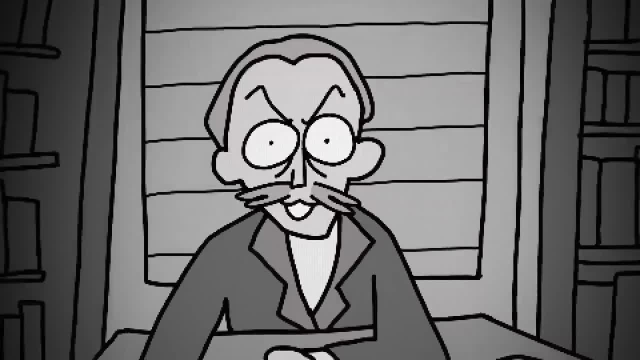 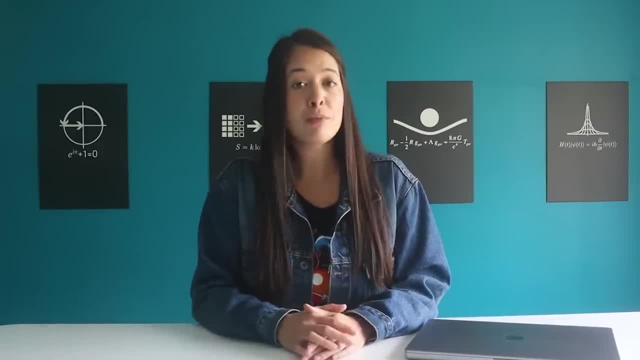 He had a dream to mechanize mathematics. Back then, mathematics was going through a rough time. Many paradoxes had shaken its foundations. The most famous one is Russell's Paradox. It's a paradox about how a computer can solve a problem. It's a paradox about how a computer can solve a 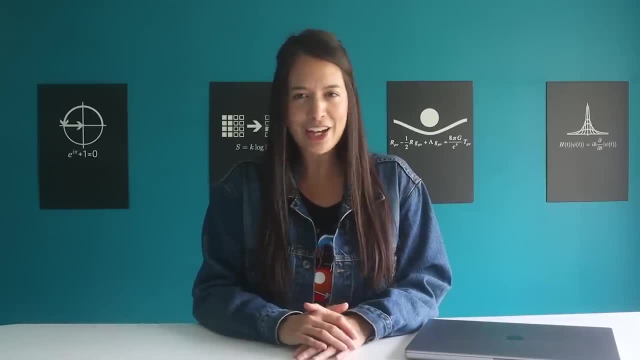 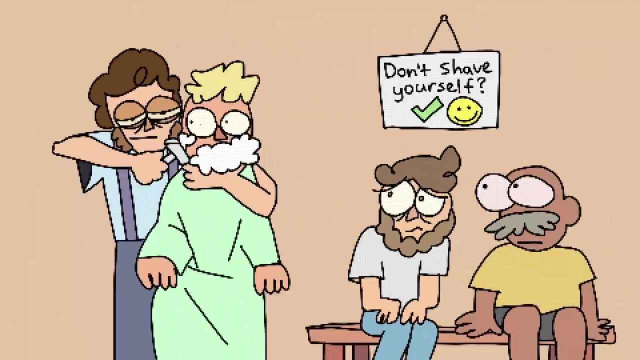 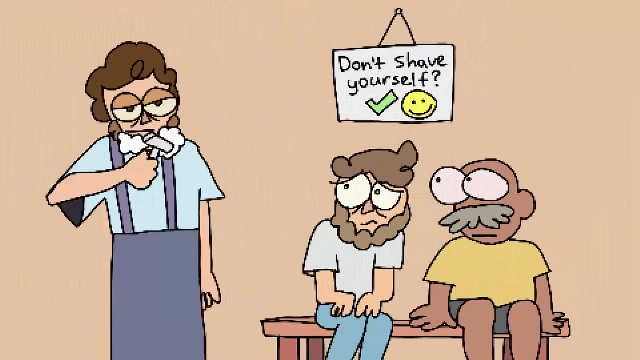 problem. It's a paradox about set theory, But the most intuitive way to understand it is actually through hairdressing. Imagine a town where there is a barber who shaves all and only men who do not shave themselves. Does the barber shave himself? If the barber does not shave himself, then he does. 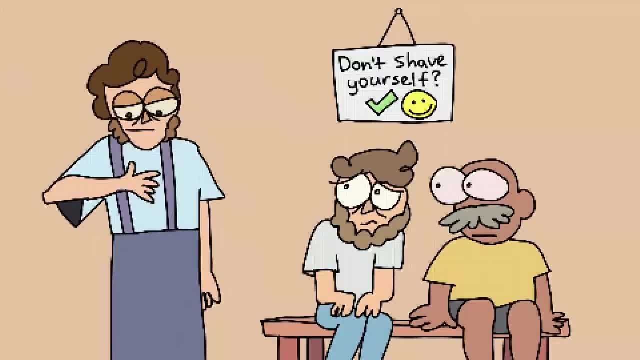 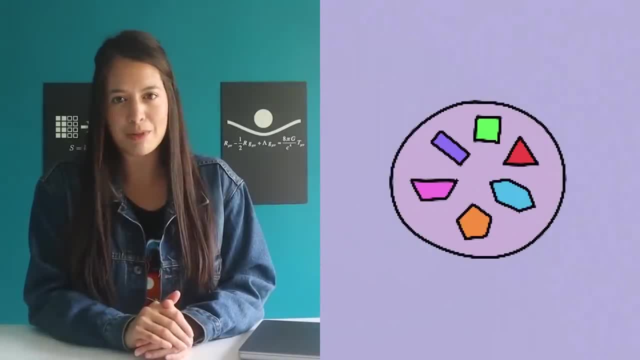 And if he does shave himself, then he doesn't. You can apply this same logic to sets. Imagine a set that contains all sets that do not contain themselves. Imagine a set that contains all sets that do not contain themselves. Imagine a set that contains all sets that do not contain themselves. 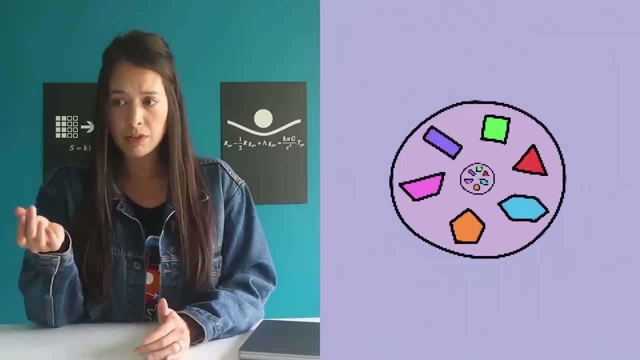 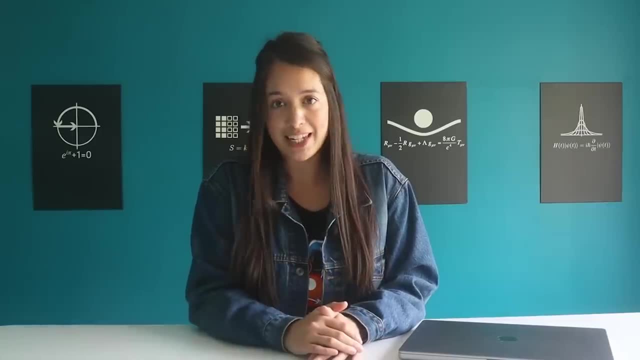 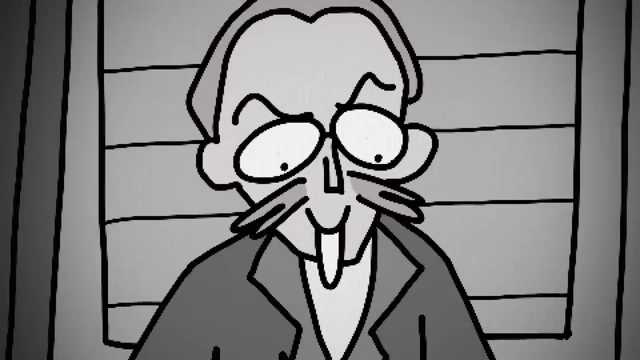 Does this set contain itself? If it does, then it doesn't, And if it doesn't, then it does. These paradoxes were not a good look for mathematics and needed to be dealt with pronto. Hilbert took it upon himself to fix this crisis. He came up with a program, Hilbert's program. 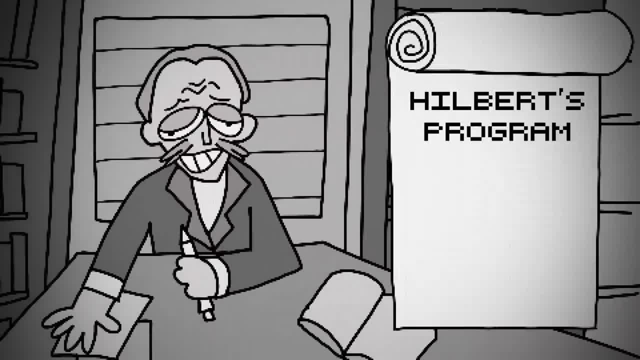 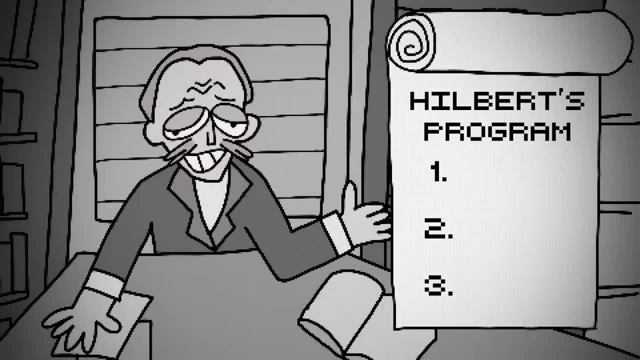 whose sole aim was to put mathematics on a firm, rigorous footing. According to Hilbert, there were three crucial questions mathematicians had to answer if mathematics was to be saved. Number one: is mathematics complete? The idea behind this question was that whatever mathematical 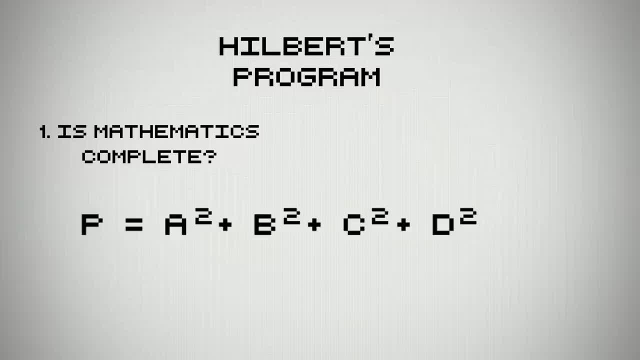 conjecture we might think of, like: every integer is the sum of four squares. we should always be able to prove or disprove it. Number two is mathematics consistent. This means that we should never be able to arrive at contradictory statements from the same set of axioms. 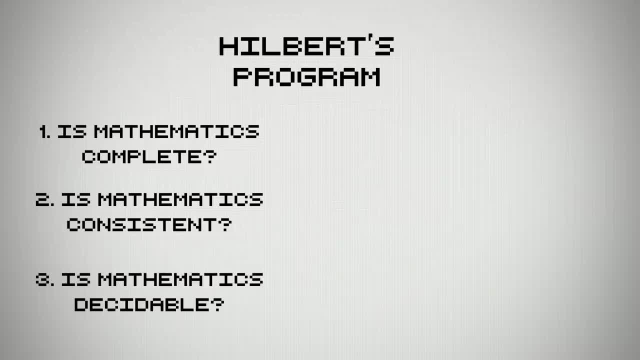 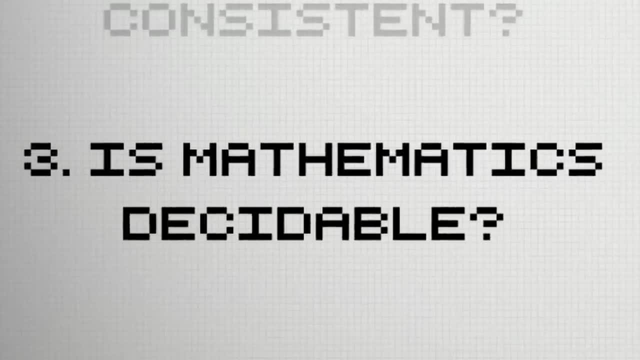 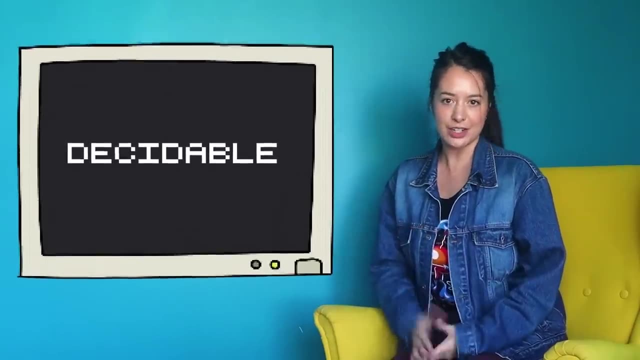 And number three is mathematics decidable. We'll come back to questions one and two later, but it's question number three that is of interest to our story. In mathematics, the word decidable means that there is a step-by-step mechanical procedure to decide whether a question has a yes or no answer, For example, 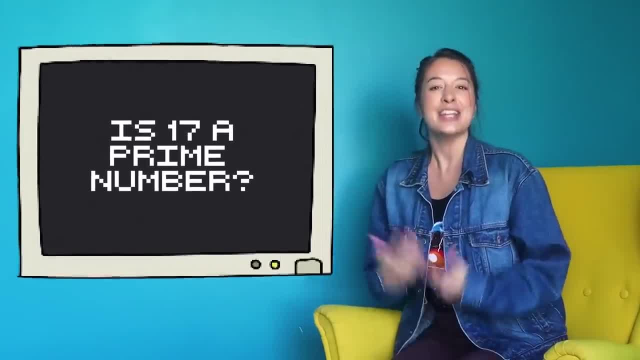 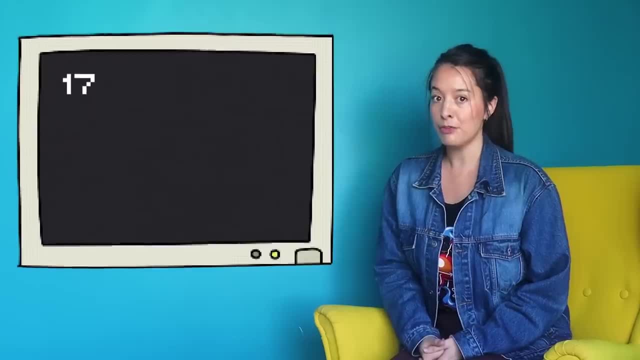 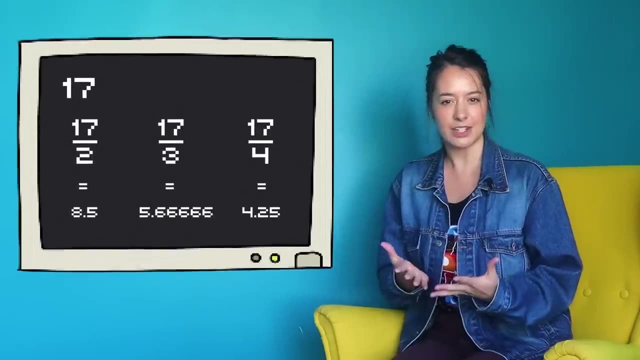 take the question: is 17 a prime number? The mechanical procedure to answer this question goes like this: Take the number 17.. For each whole number, from 2 to the square root of 17,. check if it decides 17.. If you found a divisor, 17 is not prime. If you did not find a divisor, 17 is prime. 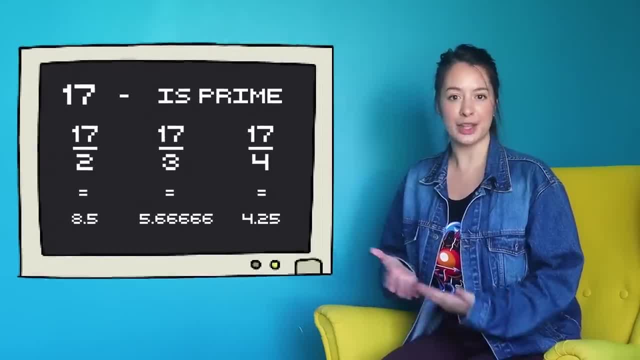 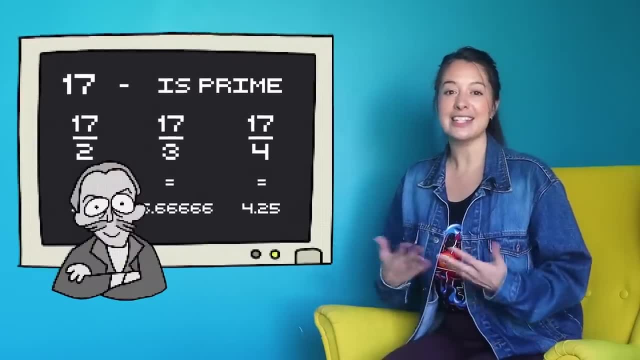 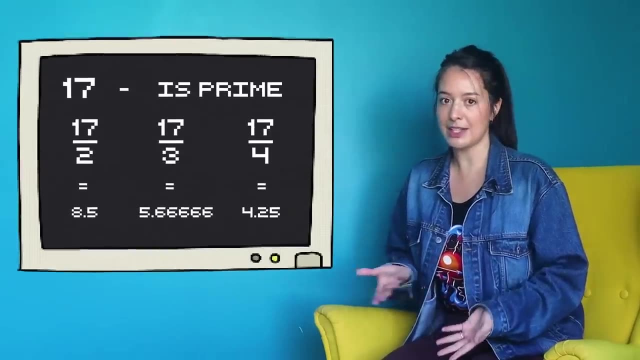 We have just used a mechanical decision procedure to answer the question of whether 17 is prime. We didn't need to think or rely on any human intuition. Hilbert called this a decision procedure, but today we would call it an algorithm. Now, if this algorithm only worked for the number 17,. 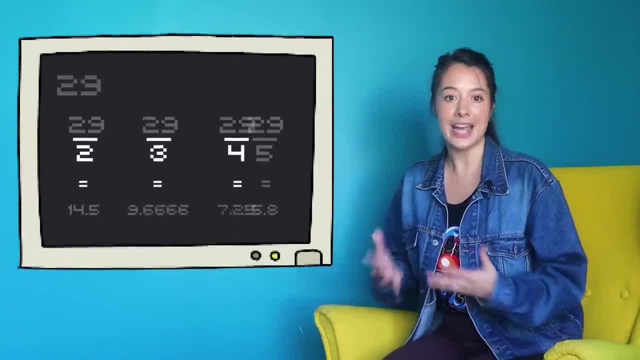 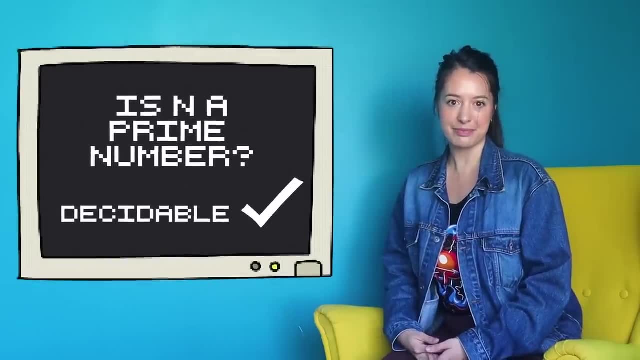 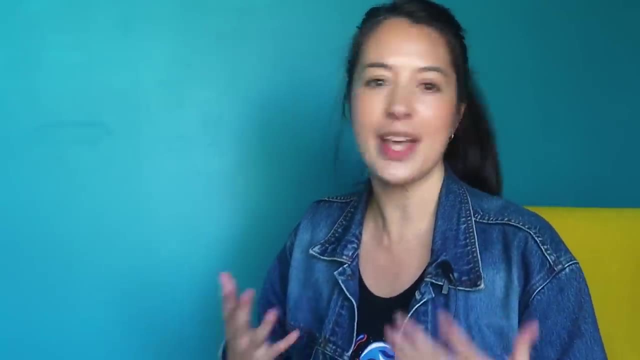 it would be pretty useless, but we can actually substitute any number and it will still work. So the question is: n a prime number is decidable? Hilbert was asking if all of mathematics is decidable. He wanted a decision procedure that could be applied. 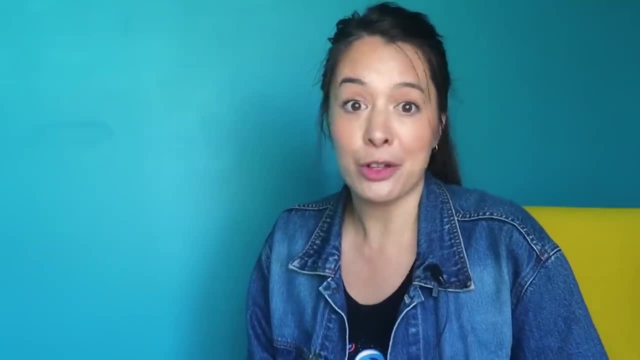 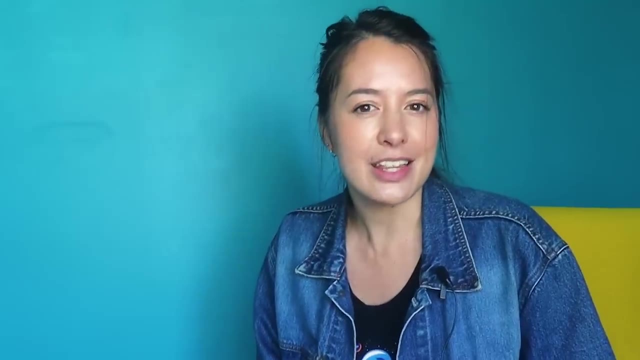 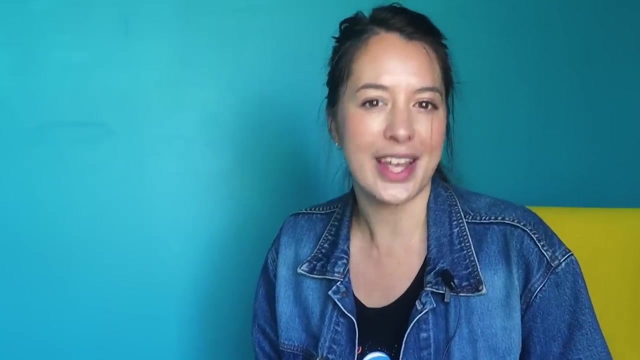 to any mathematical question. He didn't want separate algorithms for separate problems. He wanted one mega algorithm for all problems. This would be nothing less than the complete mechanization of mathematics, A magical algorithm that could answer any question with a yes or no answer. We could ask it the Riemann hypothesis: Do all non-trivial zeros of the Riemann zeta function lie on the critical line of one half? Or the Goldbach conjecture: Is every even integer greater than two the sum of two primes? 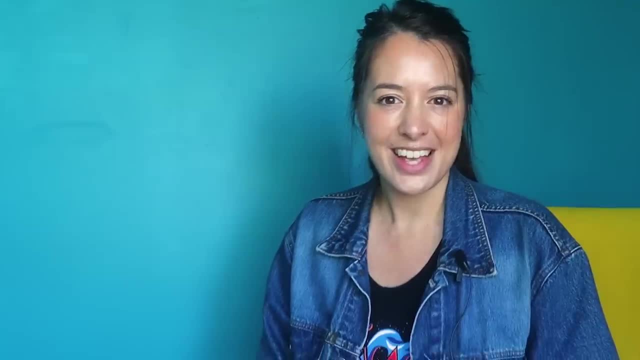 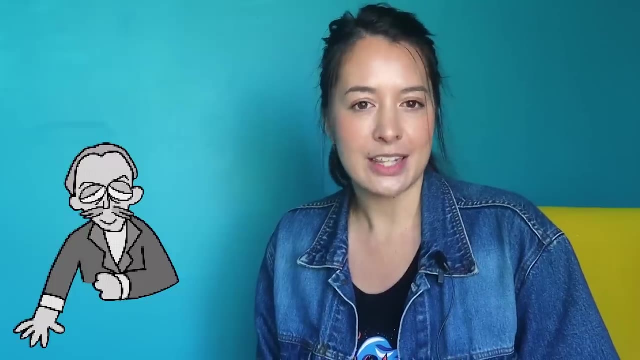 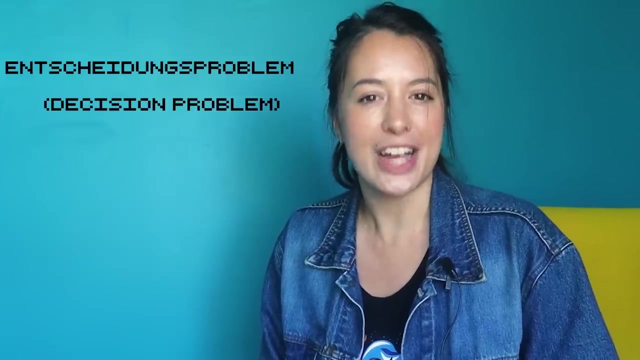 And it would run its algorithm and spit out a yes or no answer. Mathematics would be solved and mathematicians would be out of a job. Hilbert was German and he called this quest the Enscheidungsproblem, Meaning decision problem in German. It quickly became one of the most important challenges. 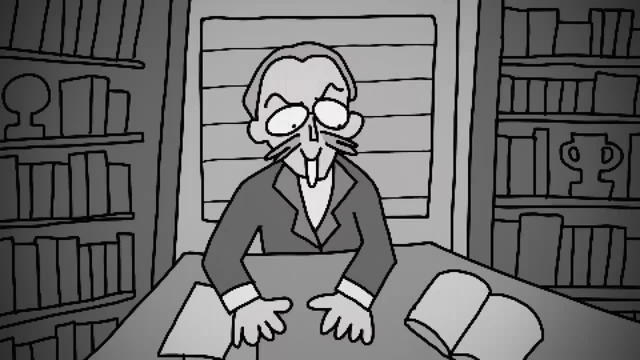 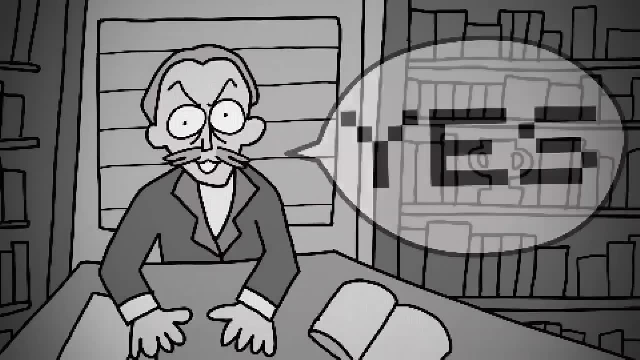 of the 20th century, Hilbert was convinced that the answer to all of his questions was yes. Yes, mathematics is complete. Yes, mathematics is consistent. Yes, mathematics is decidable. He had always been an optimist who rejected the Latin maxim. 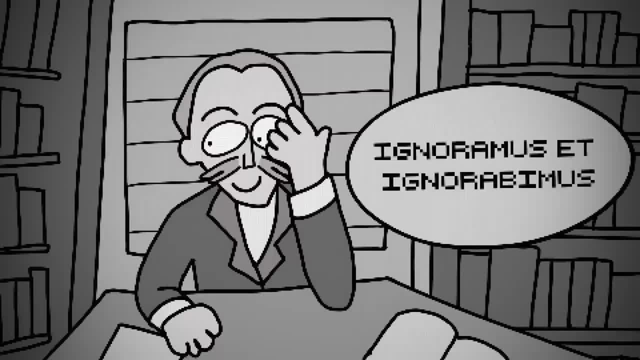 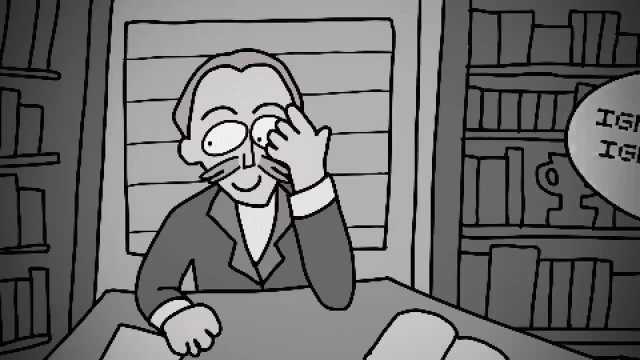 ignoramus et ignorabimus- We do not know and we will not know. This maxim represents the idea that scientifically, knowledge is limited, And Hilbert disagreed with it so much that he said: we hear within us the perpetual call: There is the problem, seek its solution. 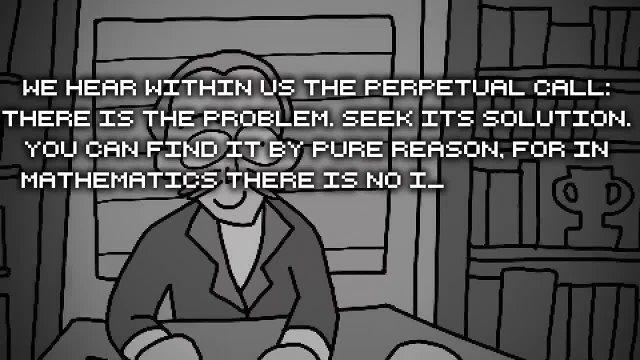 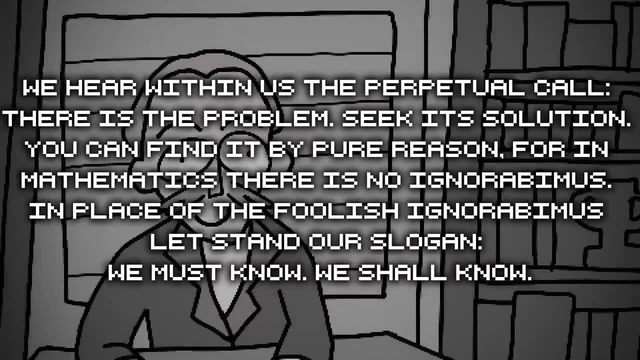 You can find it by pure reason, For in mathematics, there is no ignorabimus In place of the foolish ignorabimus. let's stand our slogan. We must know, We shall know. The last words are printed on his tombstone. 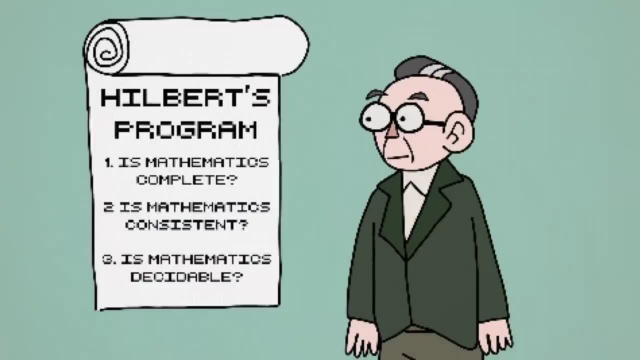 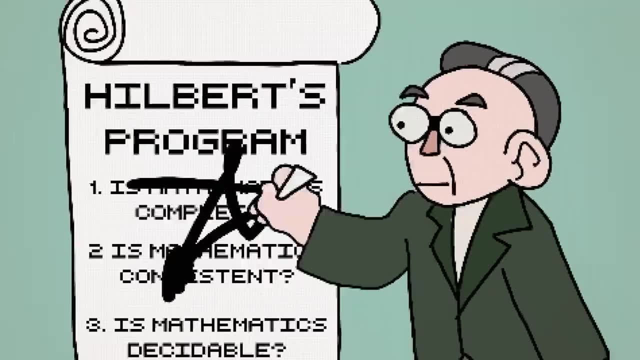 Not long after Hilbert said this, a man named Kurt Gödel came along and showed that in fact there are things we shall not know- That the first two of Hilbert's three questions were unattainable. Gödel did this via his incompleteness theorems. 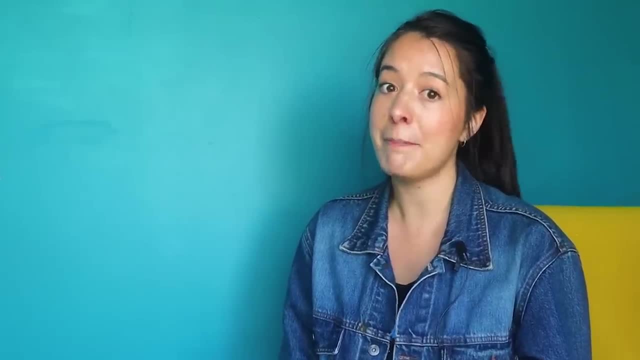 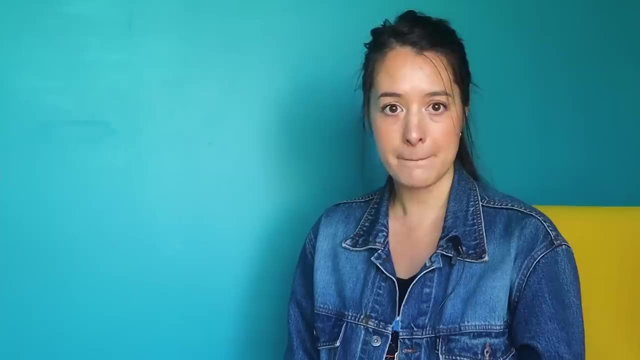 which proved that any set of mathematical axioms will inevitably be incomplete. There will always be true facts about numbers that cannot be proved by a set of starting axioms. He also showed that no powerful enough set of axioms could ever prove its own consistency. 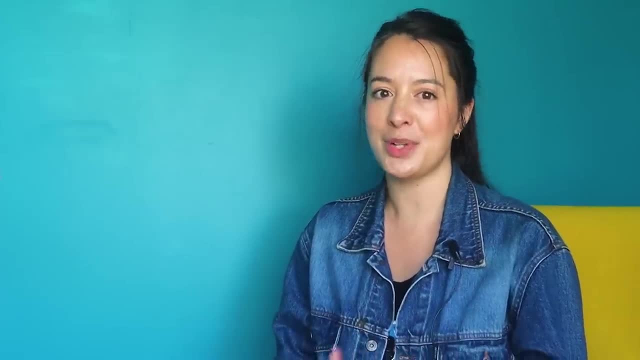 I'm making a video about Gödel's incompleteness theorem, so don't go too much into it here. I know I've been saying that for a while, but I really am. I just want to make sure that it's good. 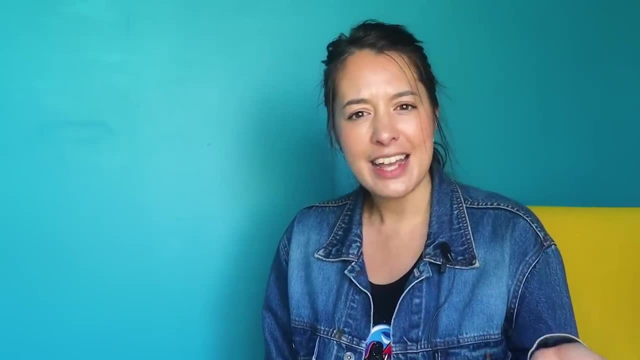 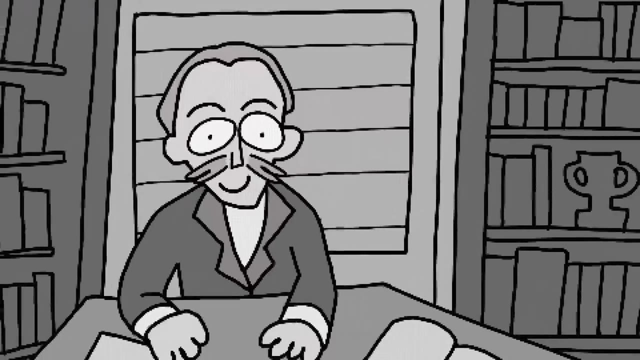 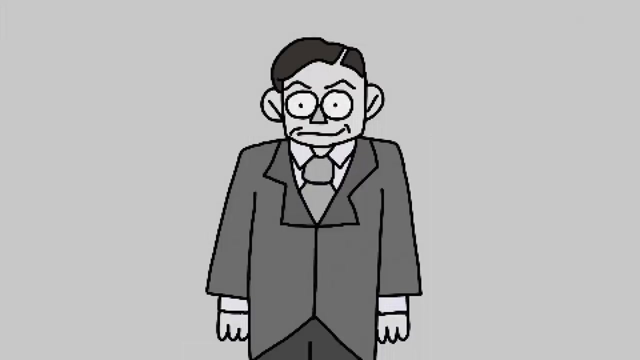 Anyway, obviously this sucked for Hilbert, But hey, at least he had question number three left, right, Right. Here the quiet hero, or villain, enters the story, A logician named Alan Turing. Turing spent his teenage years at the Chabon Public School. 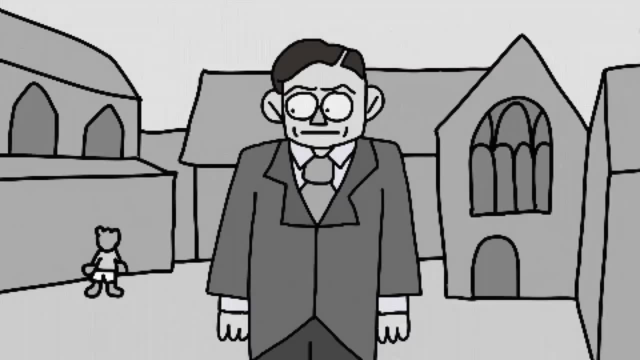 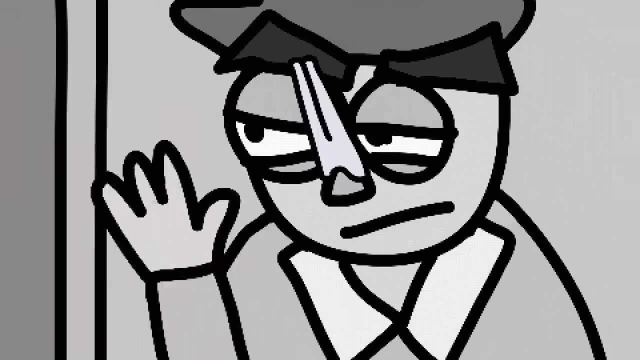 in an environment in which competitive sports were valued and mathematics was not. One of his teachers even thought of science as low and cunning and spoke of mathematics as imparting a bad smell to the room. His parents were even warned of the shame of having a son. 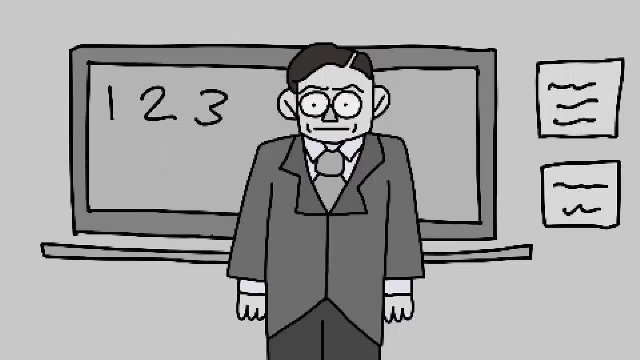 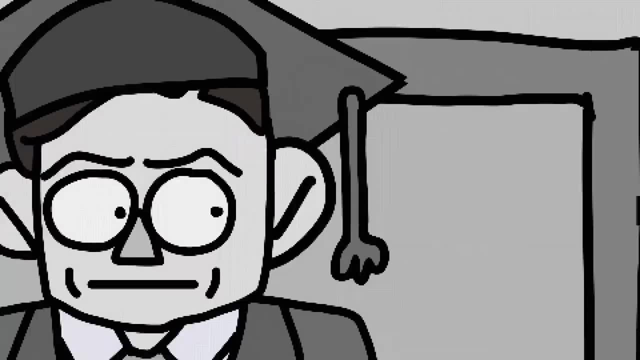 who was a mere scientific specialist. Despite all this, Turing went on to do a PhD in computer science at Princeton University, And it was here that 24-year-old Turing first heard of the n-Scheidungs problem. Turing would go on to publish what has been hailed. 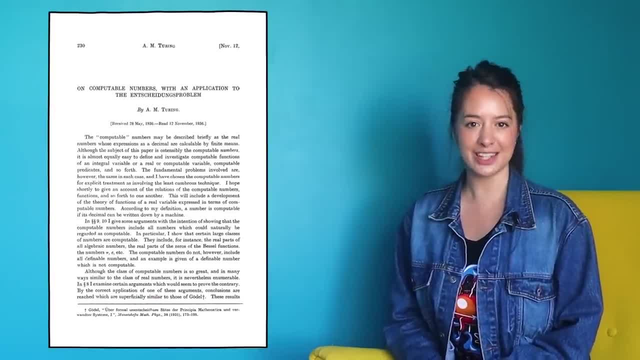 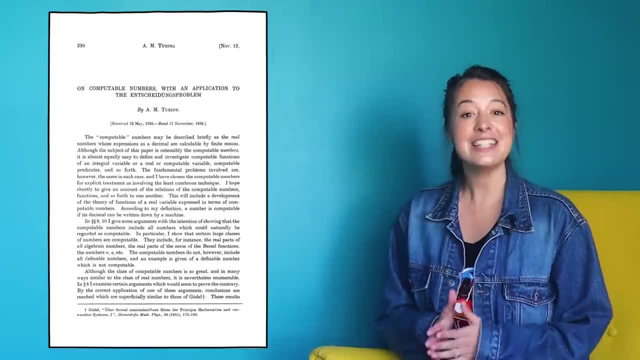 one of the top 10 science papers of the 20th century, A paper published by the University of New York, a paper called On Computable Numbers, with an Application to the n-Scheidungs Problem. In this 36-page paper, Turing kicked off the entire field of computer science. He formalized the idea of computation, defined what an algorithm was devised, the theoretical framework for universality, proved the impossibility of Hilbert's n-Scheidungs problem and revealed the limits built into computation, which stand to this day. Again, this was done before, though. 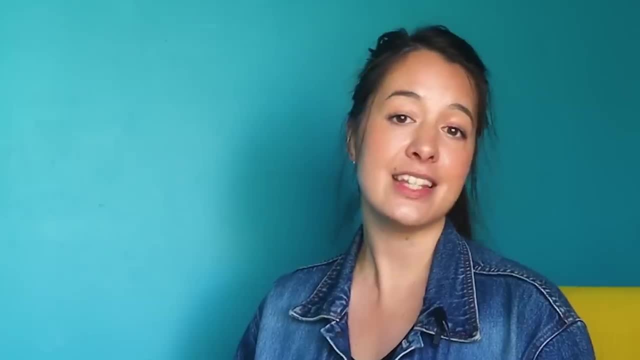 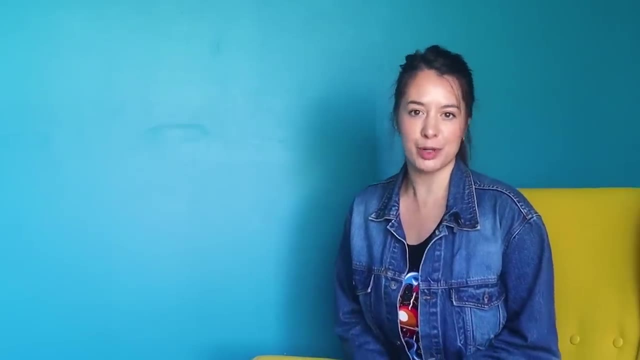 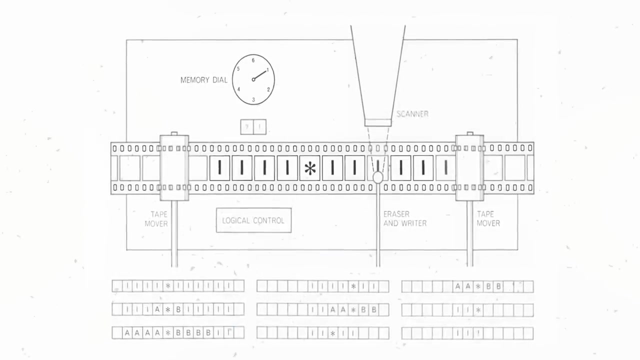 Before the first modern computer was even built. Let's see how Turing broke the last piece of Hilbert's heart. Turing demonstrated the first ever undecidable problem. He demonstrated it with his Turing machines, a slow and simple imaginary computer that he proved to be theoretically capable. 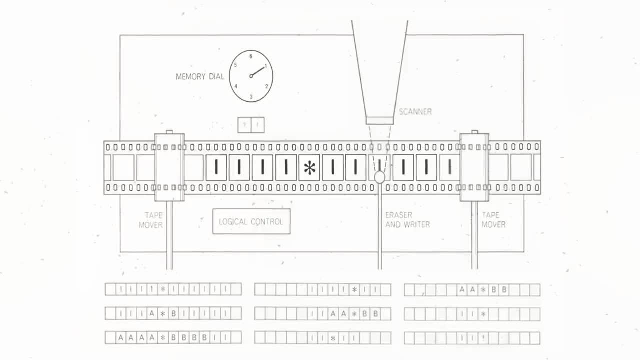 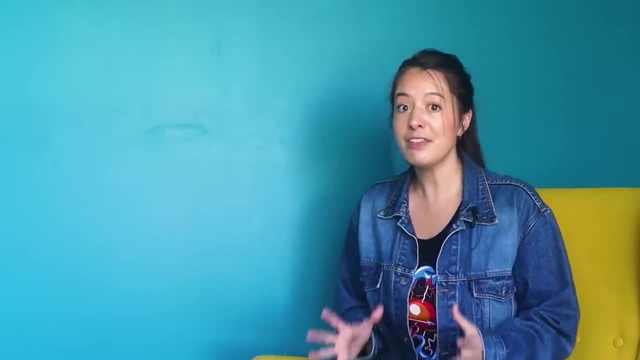 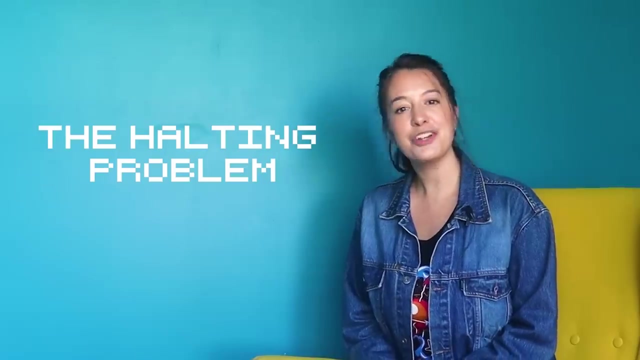 of performing all the operations of any computer. What's amazing is that, although this was written years before the first computer came into existence, all of his ideas translate perfectly to modern computer programs. His undecidable problem is called the halting problem. 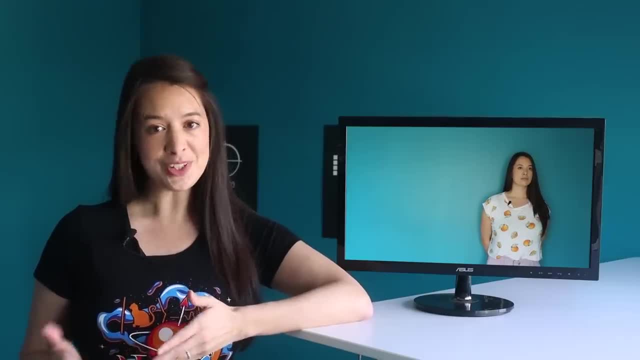 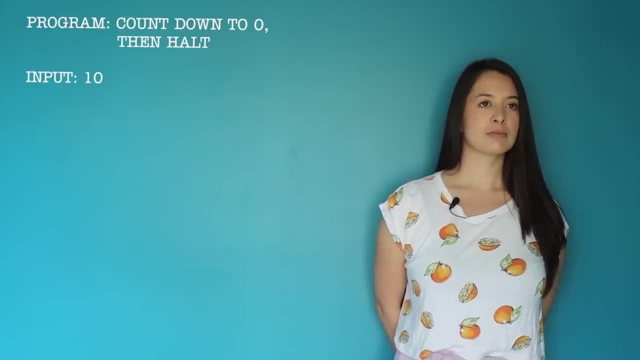 And it goes like this: Some programs halt. Take the program, count down to zero and then halt and input the number 10.. It halts when it reaches zero: 10,, 9,, 8, 7, 6,, 5,, 4, 3, 2, 1, 0. 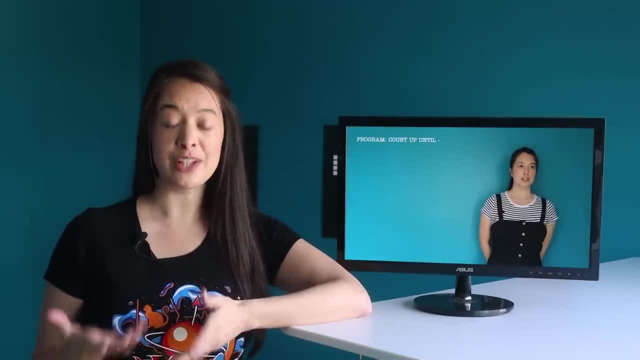 Some programs do not halt, like count up from zero until you reach minus one: 0,, 1,, 2,, 3,, 4,, 5,, 6,, 7,, 8,, 9,, 10.. This program will never halt. 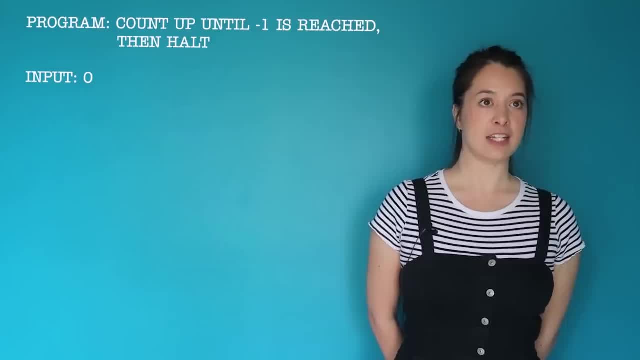 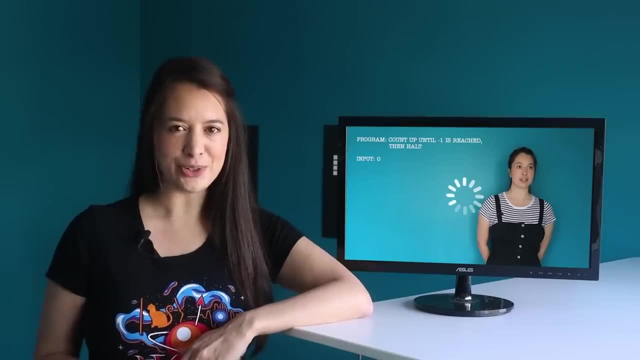 as it will never reach minus one. It will just keep going on and on forever. For some programs it's not obvious whether they will halt or not. Like you know, when your browser is frozen with that little circle, Is it about to load? in the next few seconds. 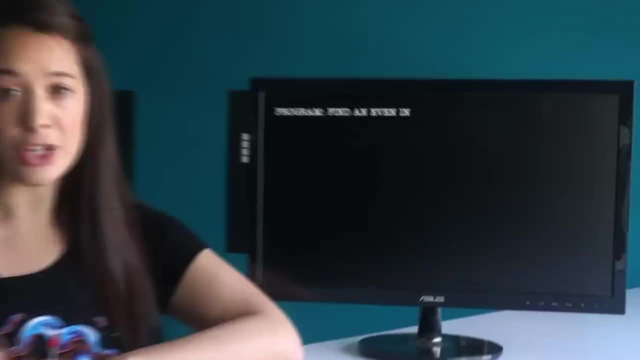 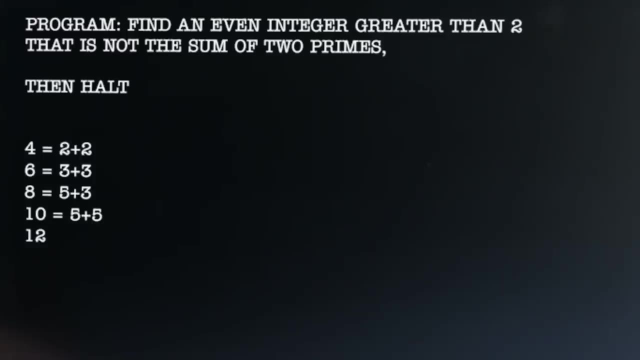 or is it stuck in an eternal loop? Or what if you wrote a program that halts when it finds an even integer greater than two that isn't the sum of two primes? Knowing whether this program will halt is the same as knowing the answer to this question. 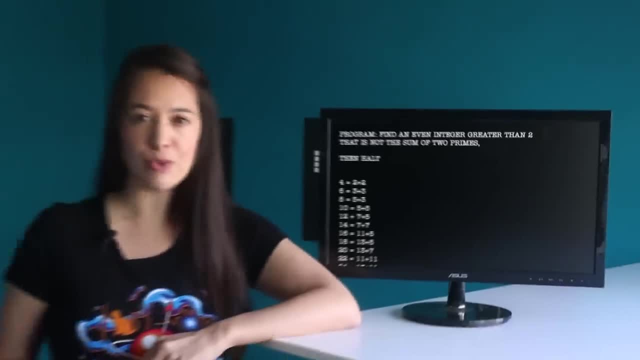 Knowing whether this program will halt is the same as knowing the answer to this question. Knowing whether this program will halt is the same as knowing the answer to this question, to the Goldbach conjecture. Wouldn't it be handy if you could write a program? 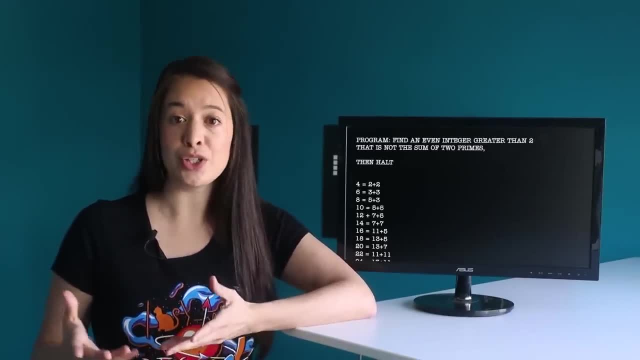 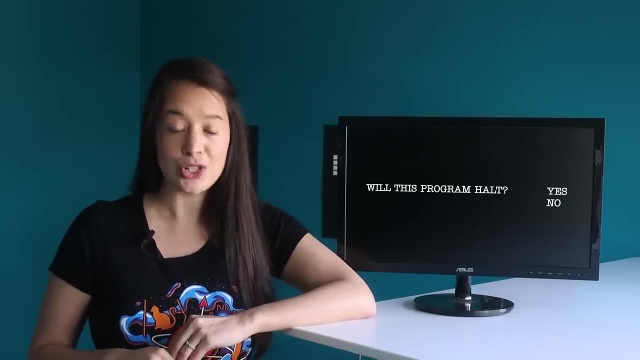 that could tell you if another program will halt. The question will this program halt? is a decision problem And, according to Hilbert, if mathematics is decidable, we should be able to answer it with a yes or no. But Turing showed this was impossible. 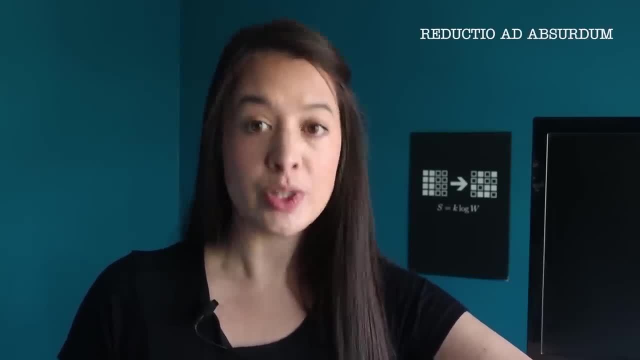 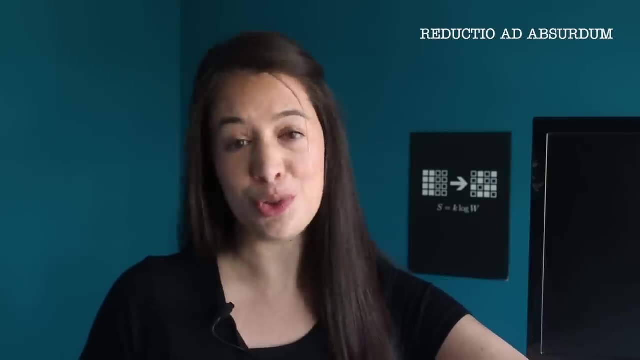 He used a proof method called reductio ad absurdum, which literally means reducing things to an absurdity. It's also known as proof by contradiction, but reductio ad absurdum sounds cooler. Here's his argument. Step one: imagine that a program does exist. 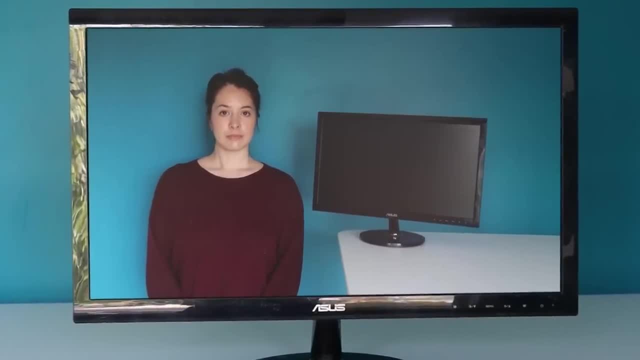 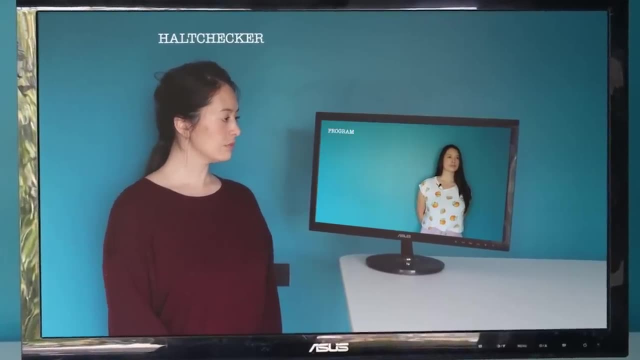 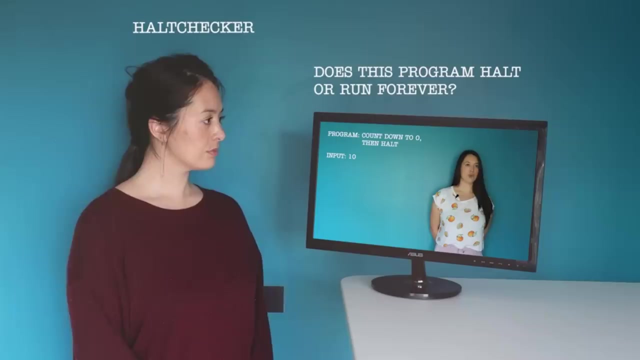 that can decide whether or not any other program and its input will halt. Call it halt checker. Give halt checker. a program and its input say this countdown program from before. Ask: does this program halt or run forever? As the countdown program clearly halts. 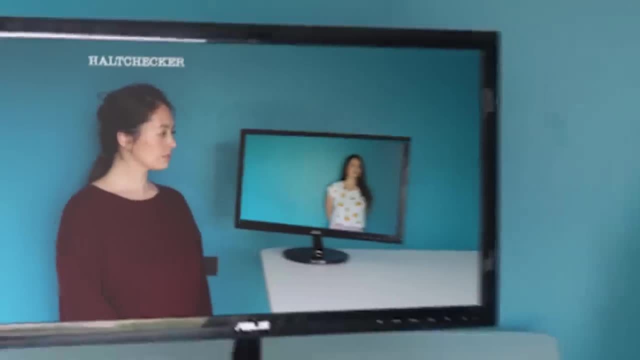 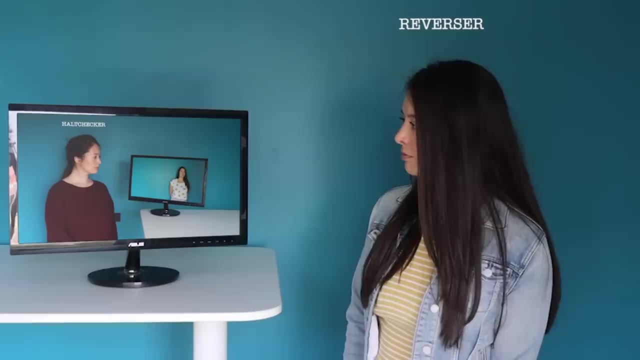 halt checker will return halt. So far, so good. So far so good. Now we create a program called reverser. Reverser looks at halt checker's output and does the opposite. So here, seeing that halt checker has returned halt. 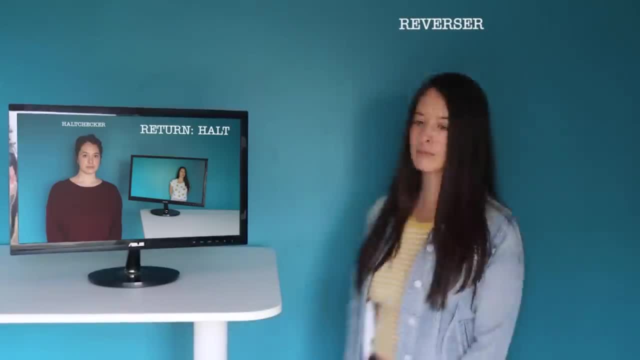 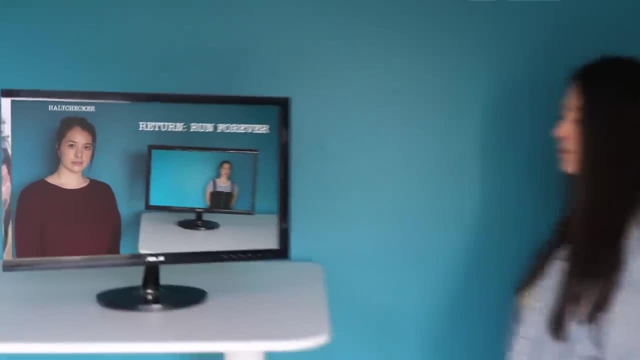 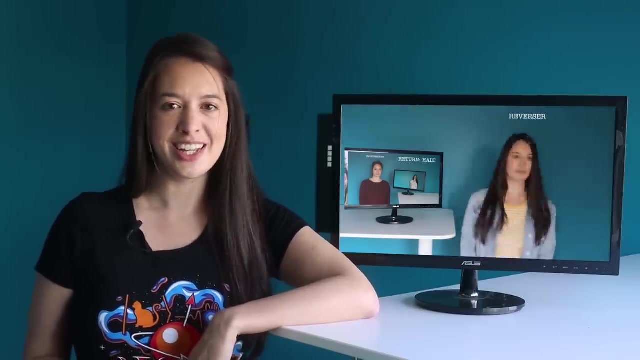 reverser runs forever. If we had given halt checker the counting up program, halt checker would have returned: run forever. and reverser would halt. Reverser is a pretty weird program, but hey, weird programs are allowed to exist in the world. 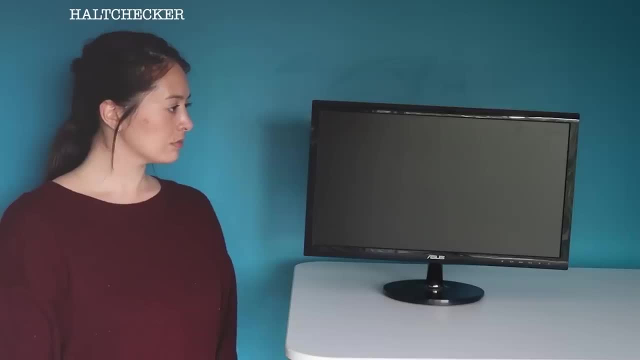 Now here comes Turing's open question, Turing's OP move. What if we give halt checker, the reverser program, as input? One of two things will happen. One reverser halts, so then halt checker returns halt and then reverser runs forever. 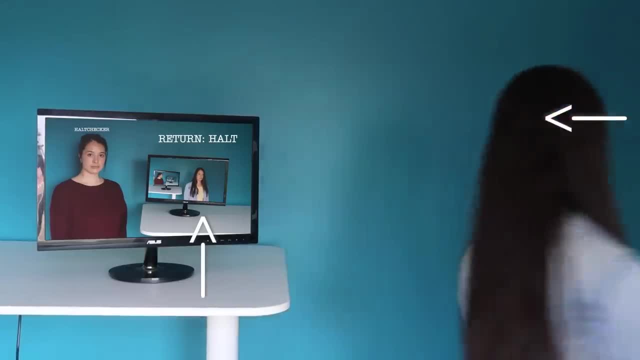 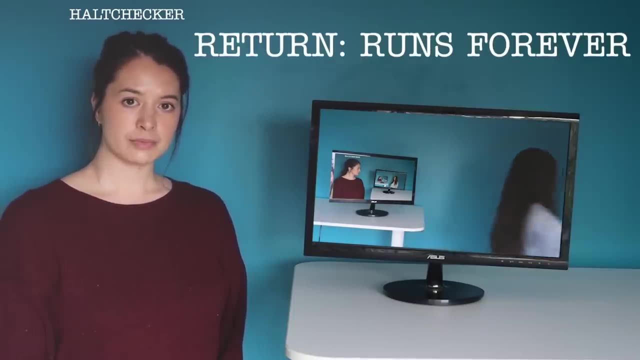 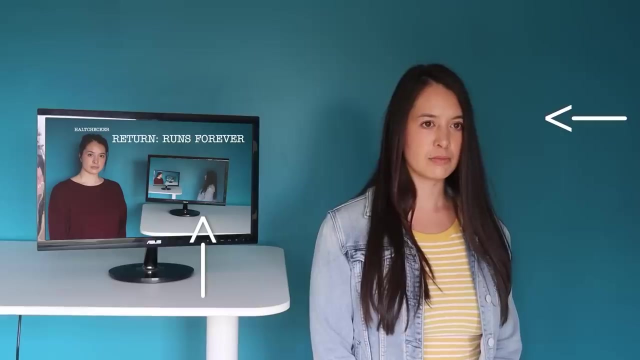 This is a contradiction, as reverser can't both halt and run forever, Or two reverser runs forever, halt checker returns runs forever and then reverser halts. This is also a contradiction for, again, reverser can't both halt and run forever. 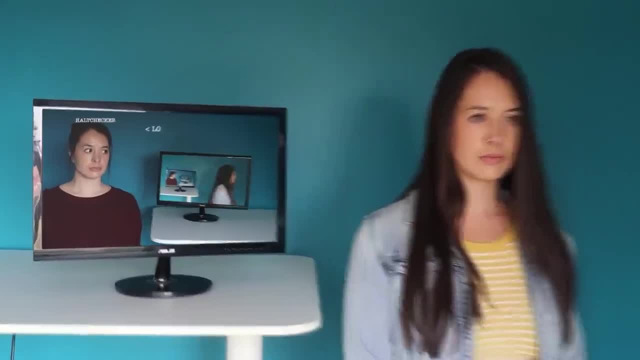 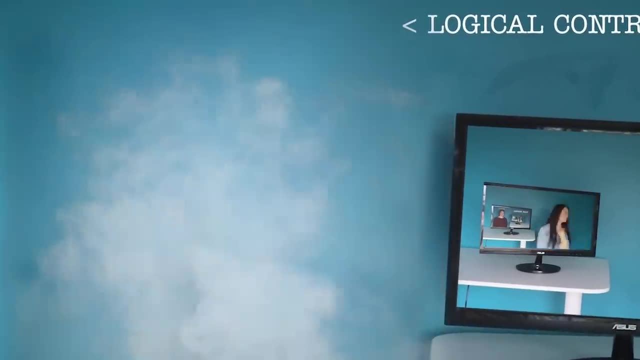 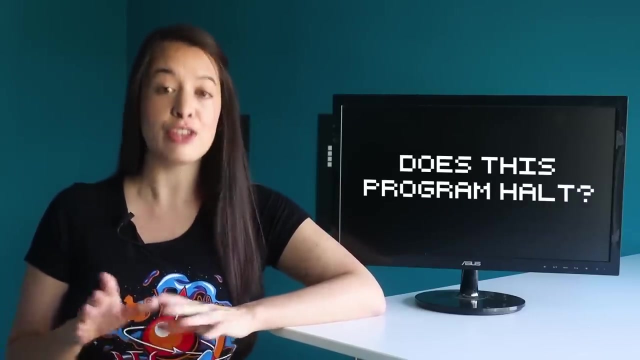 The very existence of the program halt checker has caused a logical contradiction. The only solution is that a program that can decide whether or not any program halts must not exist. So we have just found the first problem that cannot be answered by a decision procedure. 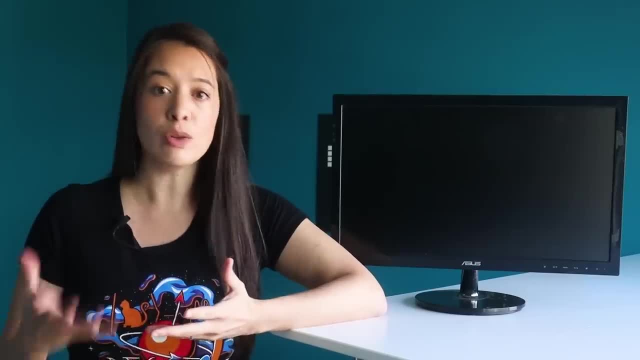 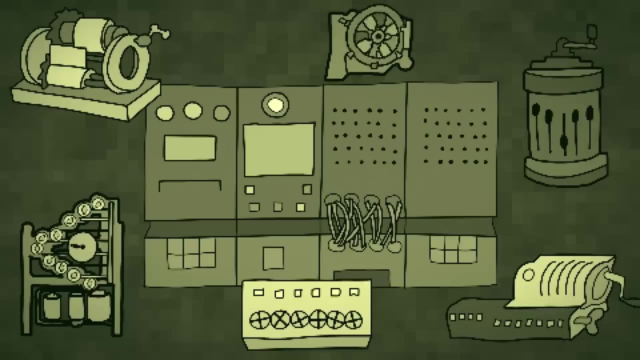 The first undecidable problem. The fact that the ultimate algorithm doesn't exist is called undecidable. Undecidability. And it's the flip side to universality, The power of universality, that a universal computer can run any and all programs. 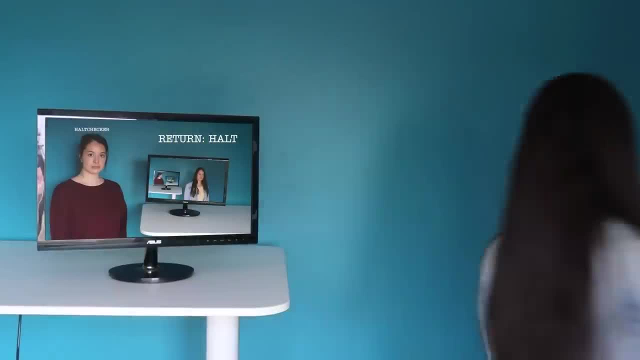 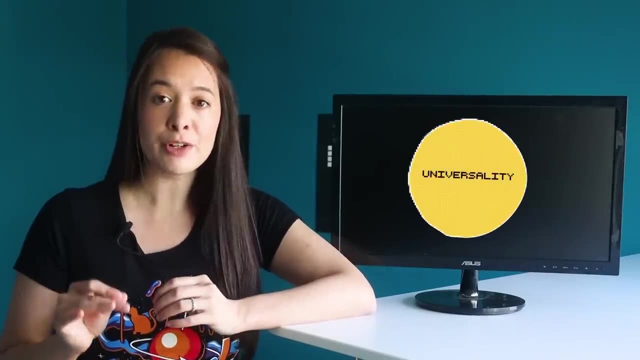 possibly run by a computer, means that we can build situations where contradictions like the halting problem have to happen. Undecidability is not a defect but an inevitable byproduct of universality. Now you might be thinking: who cares about this? 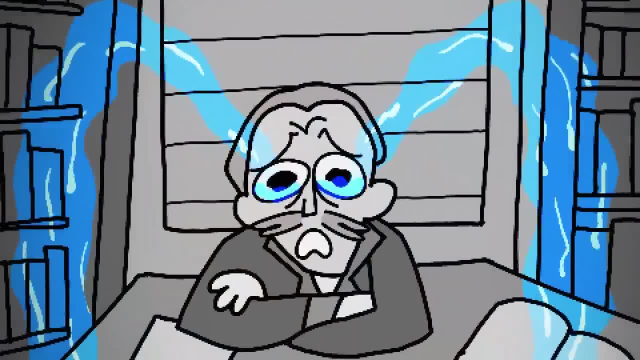 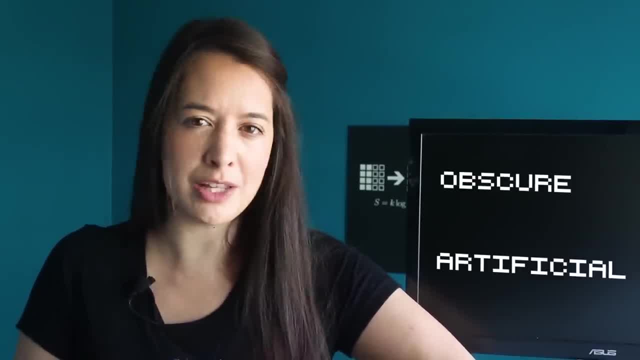 Sure, it crushed Hilbert's dream. Not every mathematical statement can be answered by some mega algorithm, But the halting problem seems like an obscure artificial problem that was made for the sole purpose of showing that mathematics is not decidable. Sure, it would be interesting to see. 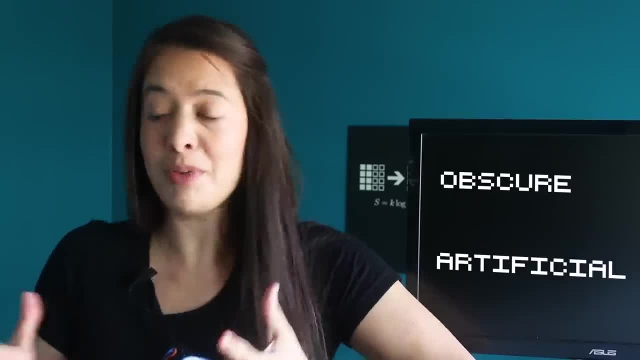 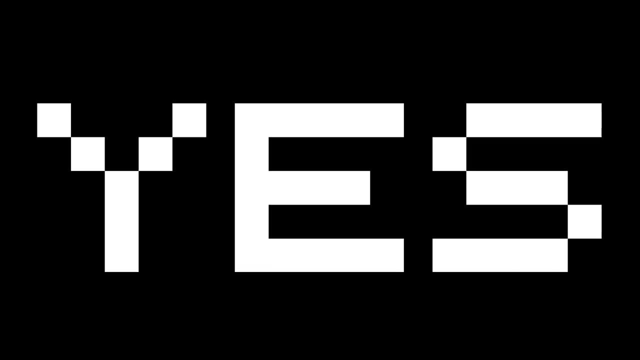 if some programs could halt. But at the end of the day, is it really such a big deal in the grand scheme of all of computation? And the answer is, unfortunately, yes. The halting problem has enormous implications for many areas of practical computing. 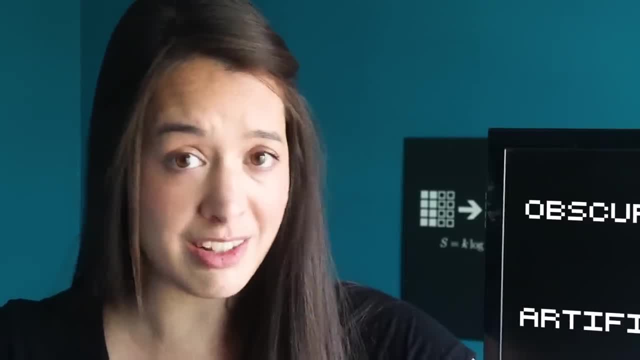 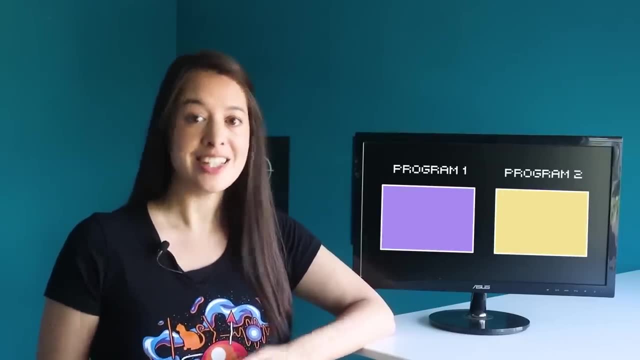 See, a lot of programming problems are really just the halting problem in disguise. So the question is: can you write a general algorithm to tell you if two programs do the same thing? It sounds simple enough, but it turns out that if you could solve this, 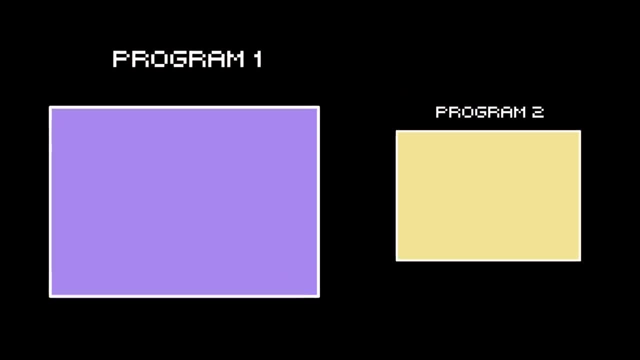 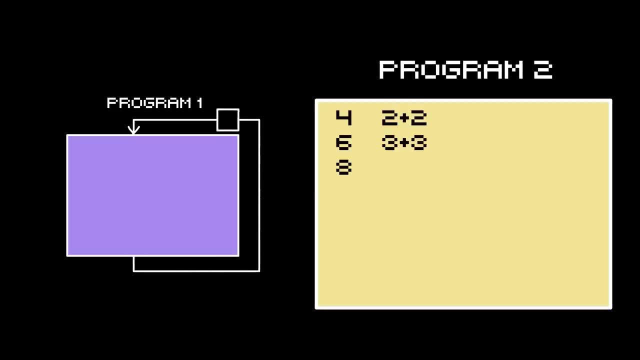 you could also solve the halting problem. You could write a program that goes into an infinite loop- a very easy thing to do. Then you could write some other program to examine every even integer and halt when it finds one that isn't the sum of two primes. 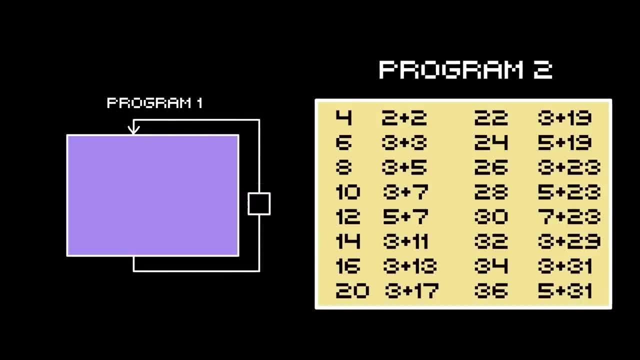 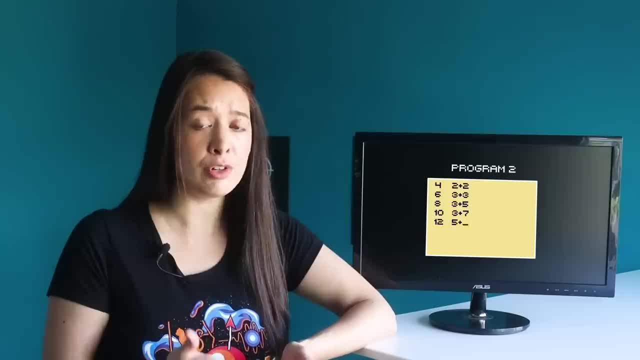 You know the Goldbach conjecture: If a program can tell you whether these two programs behave in the same way, that's effectively asking whether this program will run forever or halt, which is an answer to the halting problem. It's been shown that answering any of the following questions: 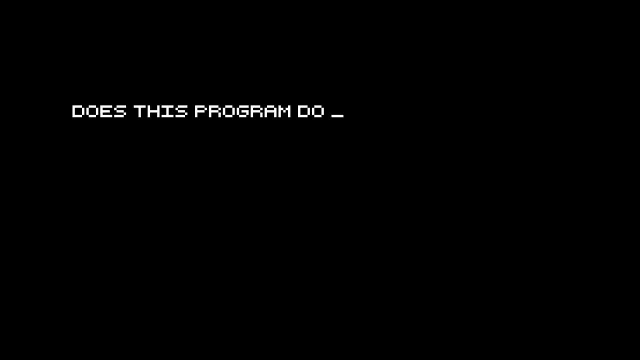 is effectively answering the halting problem. Does this program do what it says it does? Will a program always return a one? Does this program add two numbers? Can this program convert an MP3 file? Is this program a virus? Does this program modify itself? 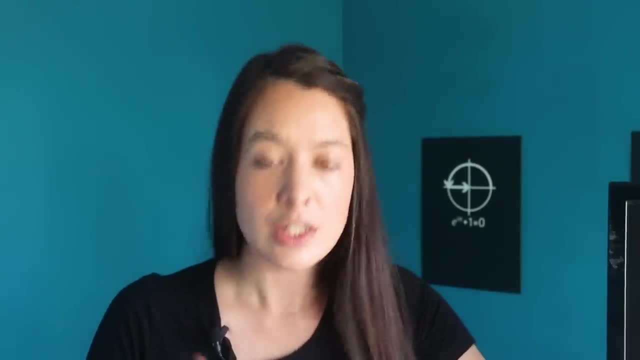 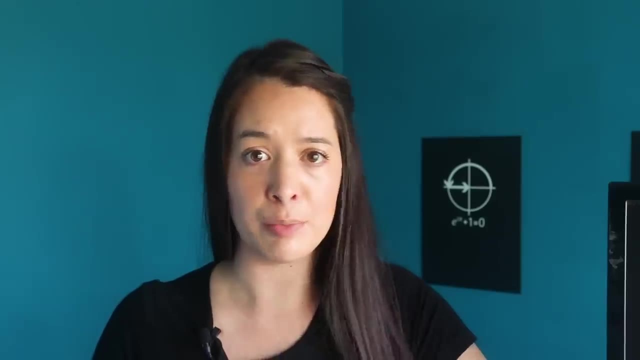 Okay, I just wanna pause here because I know there's probably some confusion. Some of you might be thinking: no, you can write a program to tell if a program returns a one. You can write a program to tell if another program adds two numbers.